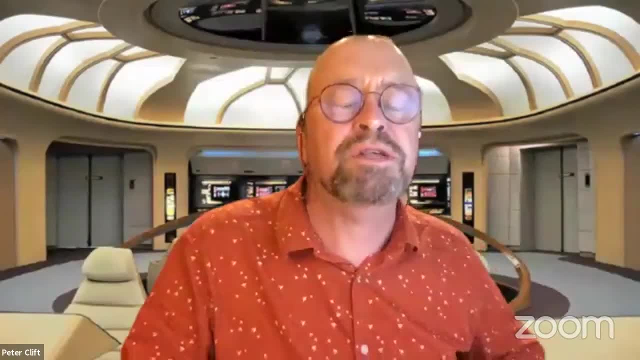 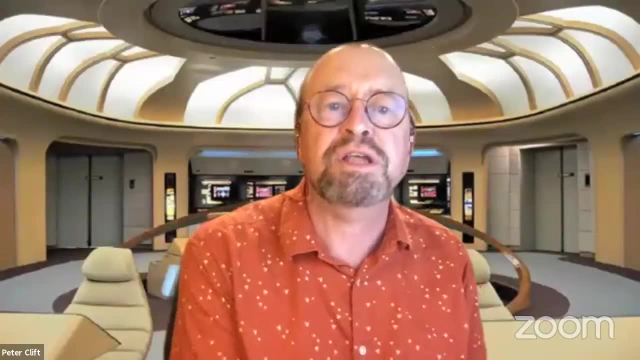 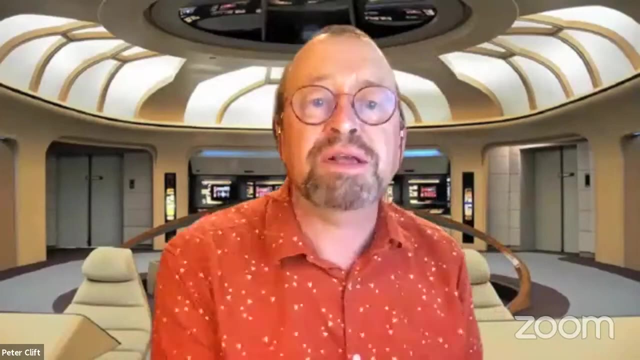 Right. So our speakers this week are Hongjin Chen and Zhao Kai Xu from the Academy of Sciences, the Institute for Oceanography in Qingdao. Zhao Kai is an old friend of mine. We were shipmates together in the Arabian Sea six years ago. 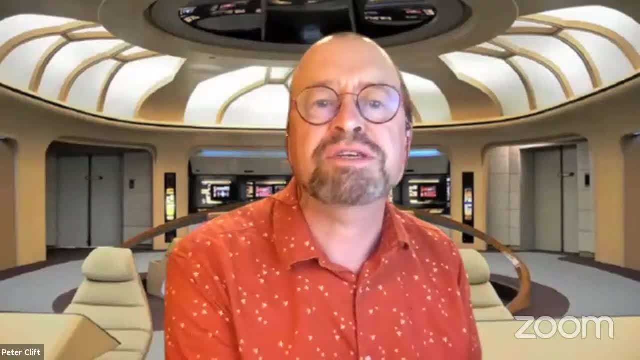 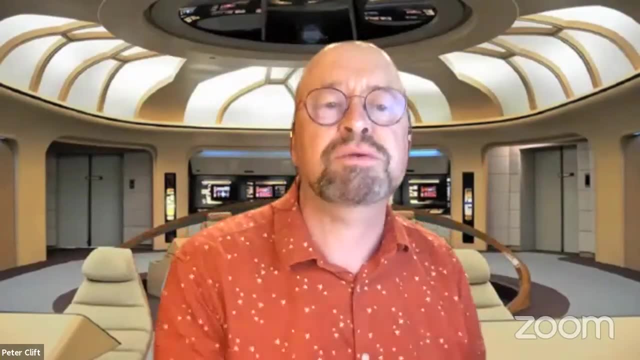 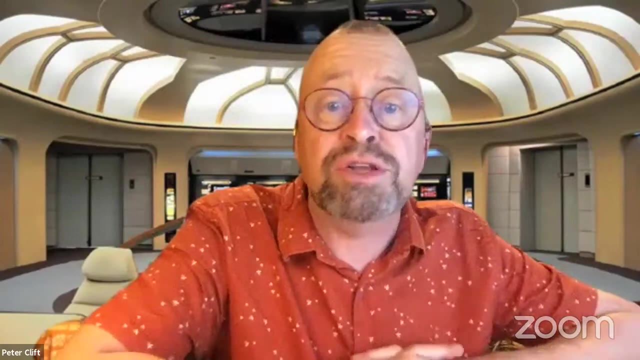 On the IODP expedition to the Arabian Sea. Zhao Kai got his bachelor's degree at the China University of Geosciences in Wuhan And he did his PhD in Qingdao on marine geology. he was a post-doc and visiting scientist there. 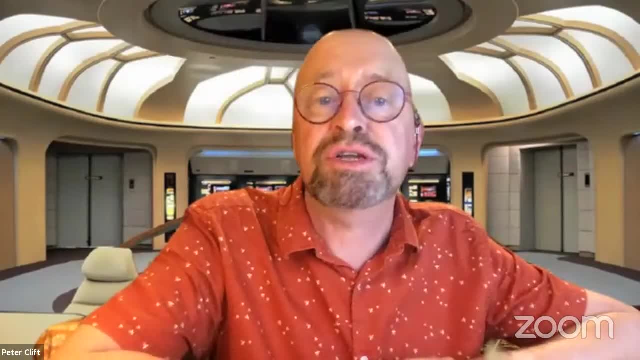 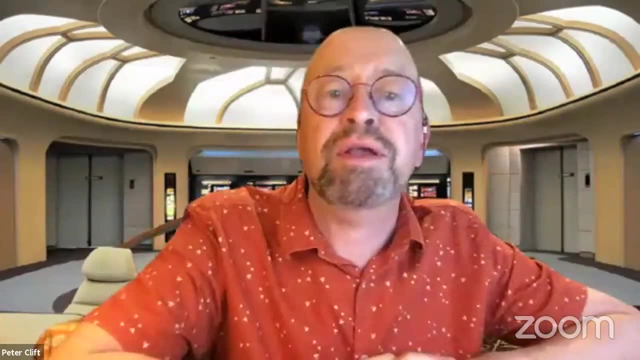 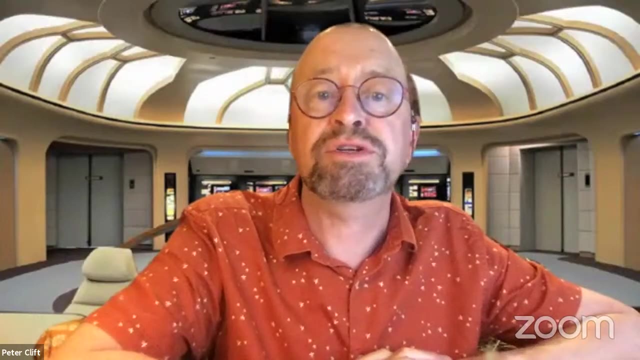 And he's worked on several IODP expeditions. as an expert on the Asian and Australian monsoons, Hong Jin got her bachelor's degree at the China University of Geosciences in Beijing before she moved to Qingdao herself for a master's degree. 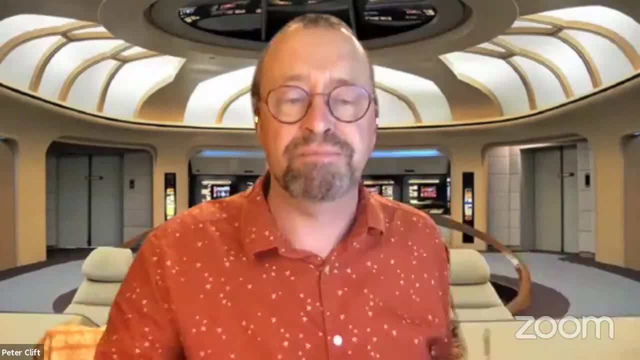 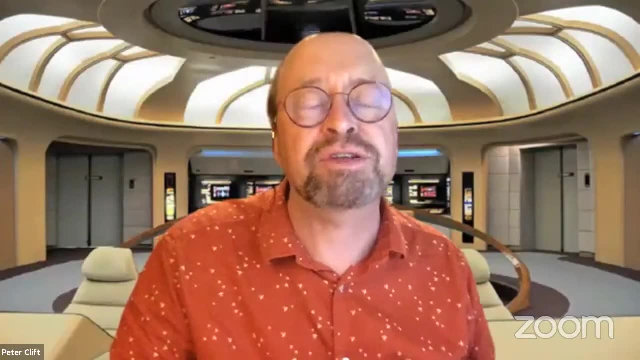 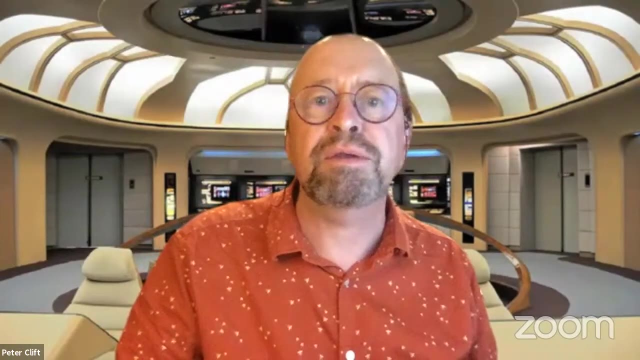 And she's now a PhD student at the Institute of Oceanography, And she worked with Zhao Kai on matters related to the Asian monsoon. So, without further ado, I will turn over the show to Oh hang about, I have to make you guys co-hosts. 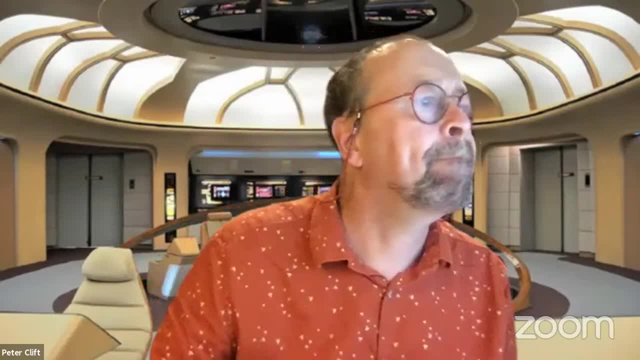 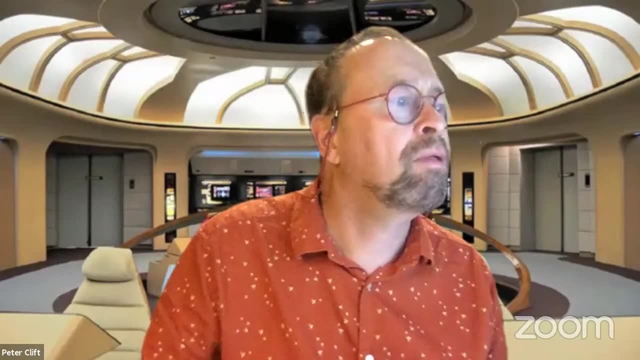 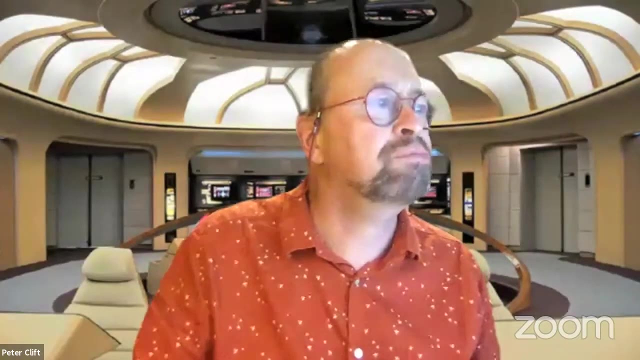 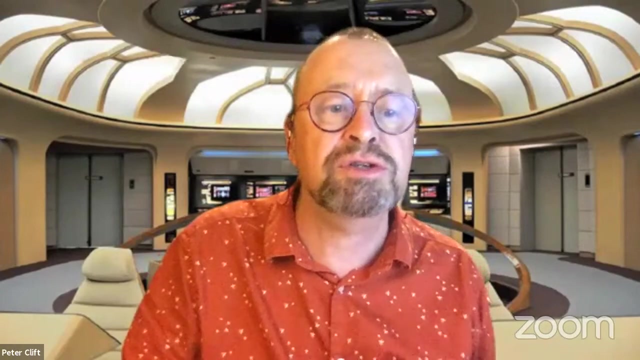 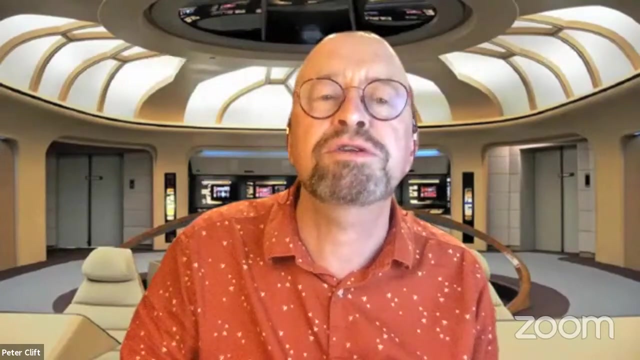 Thank you so much, And that should be good. So now I I would like to ask maybe if people could mute and sign into your videos. And I don't know which of you is going to start the talk. Hong Jin, are you going to be starting? 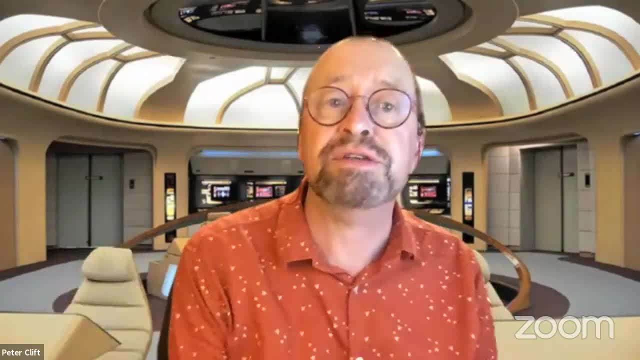 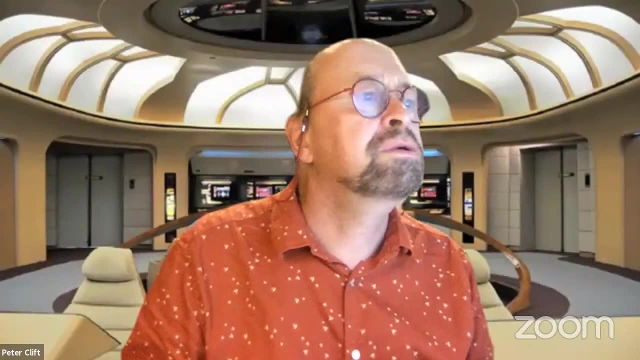 Yes, yes, yes, Great, Or you should be able to share your screen. Okay, I'll share my screen now. That's great. You're going to talk to us about enhanced indigenous input into the tropical Pacific and Indian oceans. 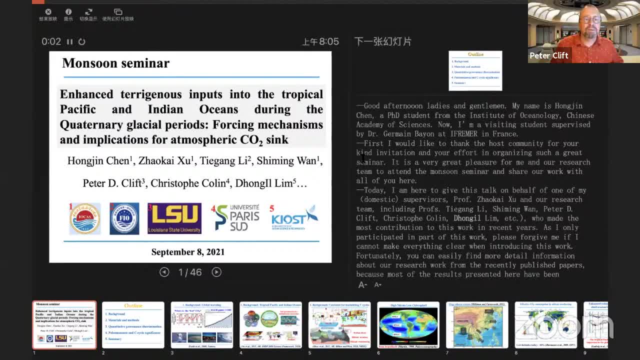 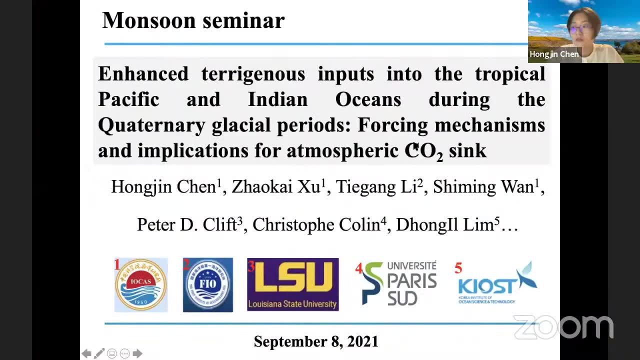 Thank you very much. Can you see my screen now? Yeah, I can. I am I Your split screen? You want to share the other screen? Yes, that's perfect. That's good. I might need to Wait a moment. 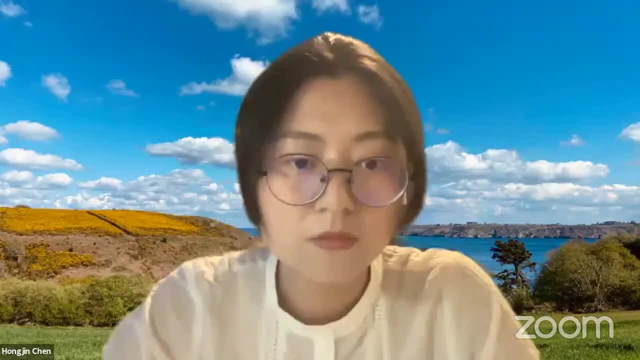 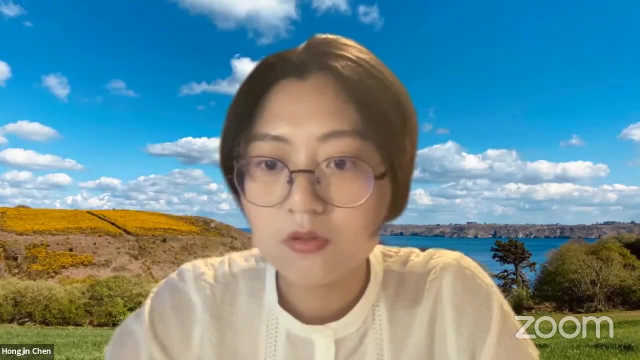 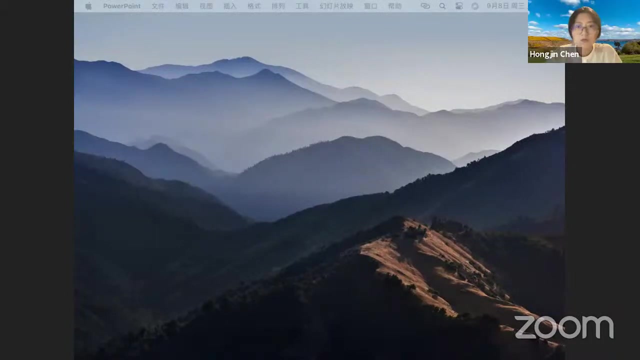 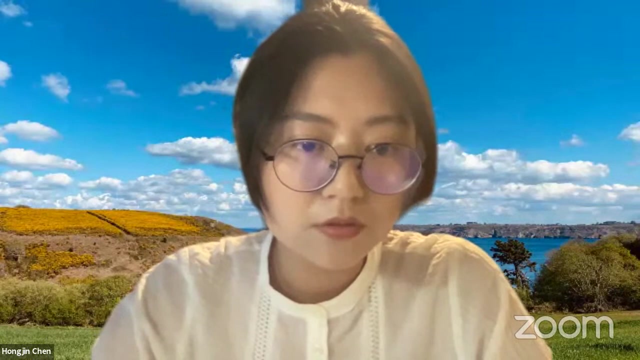 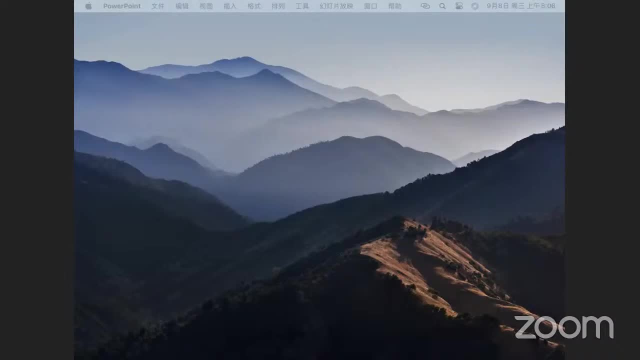 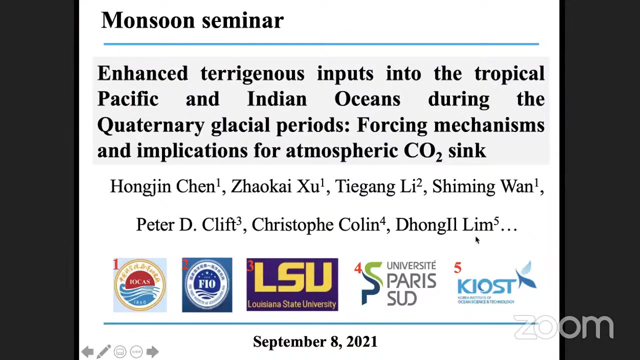 Okay, Which screen can you see? I cannot, I just see some mountains like a blind screen. Now we see your sort of split screen There. perfect, That's it Very good. Thank you so much. Sorry about this. 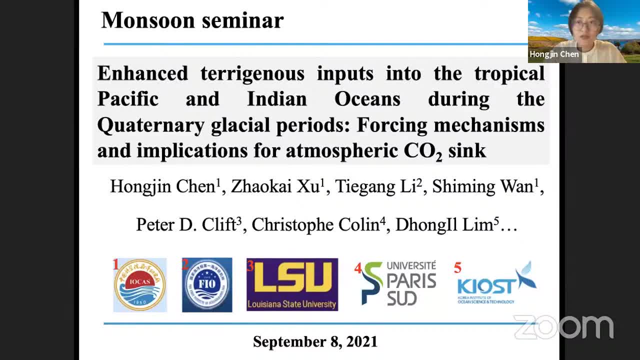 It's okay. Okay, I'll start now. Yes, please, Okay, okay, Thank you. So good morning, good afternoon and probably good evening, ladies and gentlemen, wherever you are. My name is Hongxin Chen. I am actually a PhD student from the Institute of Oceanology Chinese Academy of Sciences. 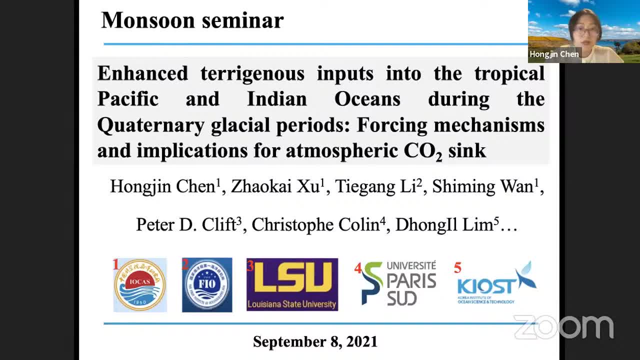 Now I am a visiting student supervised by Dr Jacques Marbain at IFREMER in France. First, I would like to thank the host community for your kind invitation and your effort in organizing such an amazing seminar. It is a very great pleasure for me and our research team to attend the Monsoon Seminar. 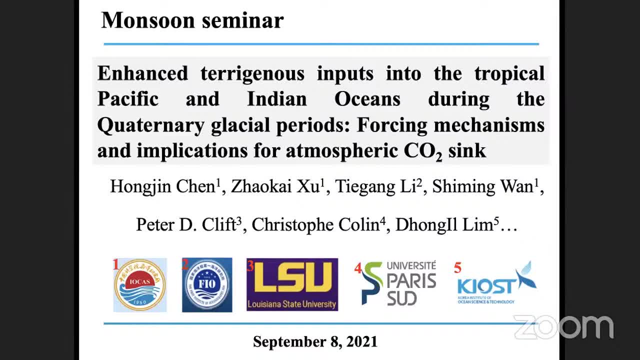 and share our work with all of you here. I'm here today to give this talk on behalf of one of my supervisor, Professor Zhao Kaixu, and our research team, including Professor Tiegang Li, Shimin Wang, Peter Clift, Christophe. 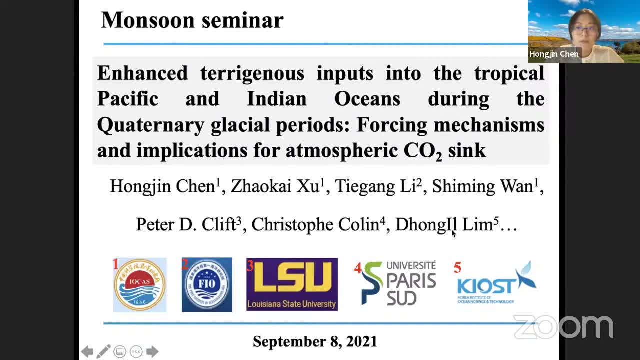 Collin, Dongyi Lin, et cetera, who actually made the most contribution to this work in recent years. As I only participated in part of this work, so please forgive me if I cannot make everything clear when introducing this work, But fortunately, you can easily find more detailed information about our research work. 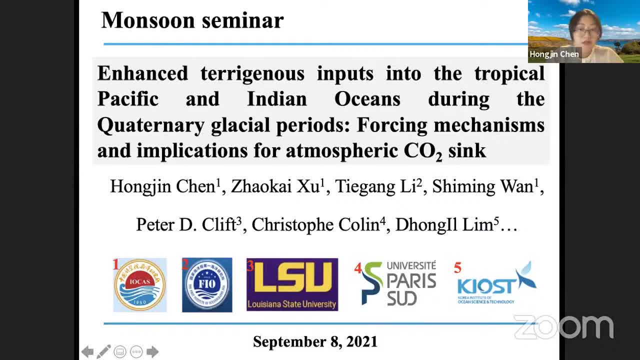 from the recently published papers and because most of the results presented here have been published. Also, if you have any questions, I'm sure my supervisor, who is also in this meeting room, would be willing to help me, And I will be happy to answer the questions at the end of this presentation. 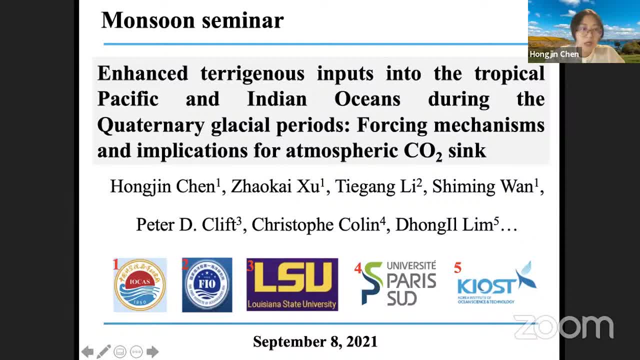 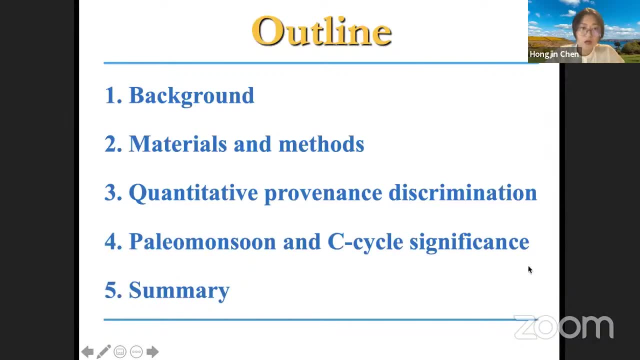 So the topic of my presentation today is enhanced terrestrial input into the tropical, Pacific and Indian oceans during the Quaternary Glacial Periods: forcing mechanisms and implications for atmospheric CO2 sink. So, as you can see here, our presentation will be divided into the following five parts. including the background information material and technical information. The first part will be a summary of the presentation and the second part will be a summary of the presentation, including the background information material and technical information. The first part will be a summary of the presentation and the second part will be a summary of the presentation, including the background, information material and technical information. 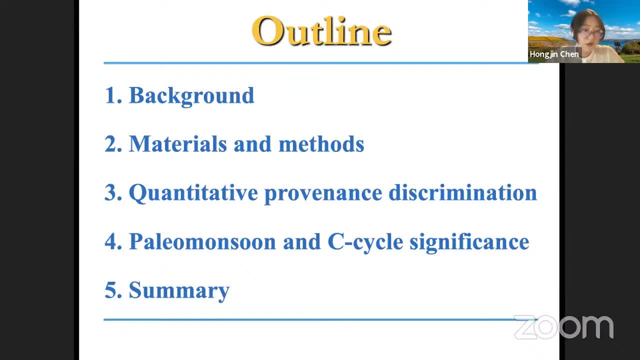 The second part will be a summary of the presentation and the third part will be a summary of the presentation, including the background information, material and technical information, And then I will talk about the quantitative provenance discrimination and the evolution of pernil monsoon and its significance for the global carbon cycle. and then the summary. 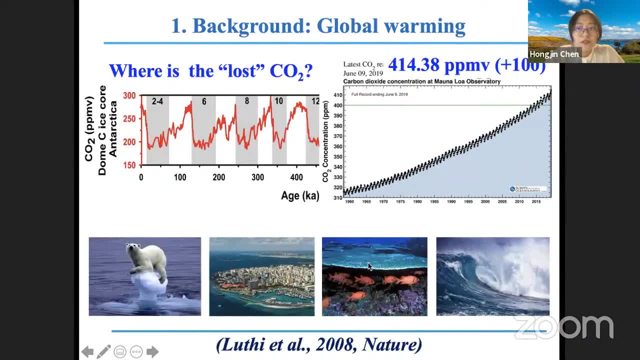 So, first of all, I'd like to start by briefly reviewing some background information. As we know, the rise of the industrialization in the last two centuries has led to a dramatic increase in the greenhouse gas, CO2 level From burning of fossil fuels, which, in turn, has led to a significant global warming. 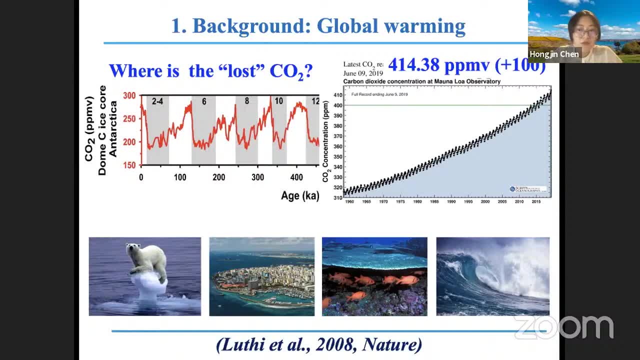 The global warming could profoundly impact human life as a result of a consequent global sea level rise, more numerous and powerful hurricanes and ocean acidification, etc. Over glacial and interglacial timescales, the Earth's past climate has been closely coupled with. 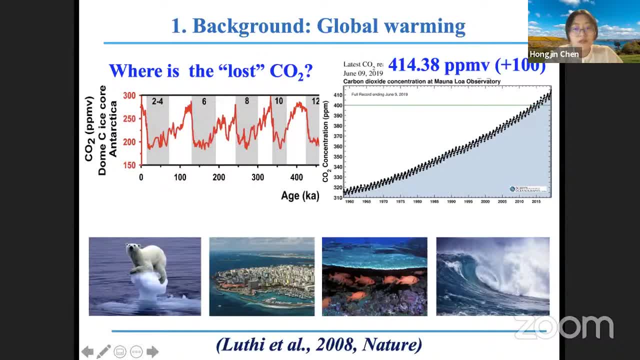 atmospheric CO2 levels since at least 800,000 years, which is a significant increase in the global warming of the atmosphere, characterized by high concentrations of CO2 during the warm interglacial intervals, by venues lower during the maxima glaciation. The carbon taken from the atmosphere during the glacial times ended up in the deep ocean. 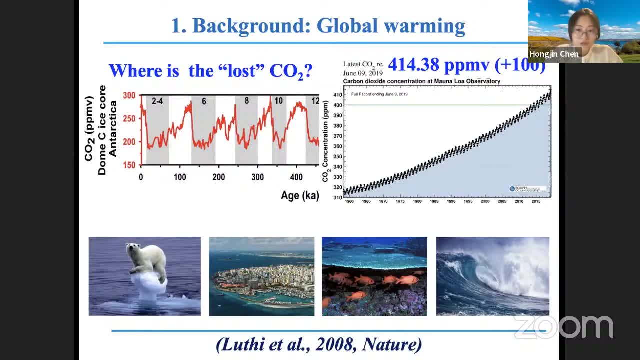 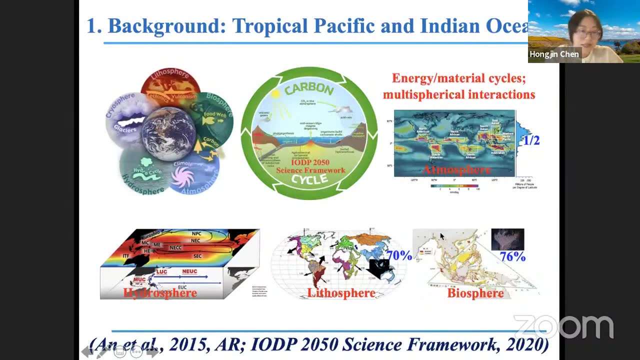 as marine sediments are an important reservoir for the global organic carbon. However, the detailed processes responsible for this transfer are still being explored. Understanding the key natural processes controlling the sinks and sources of the carbon and how they are changing are essential to understanding how carbon concentrations in the atmosphere 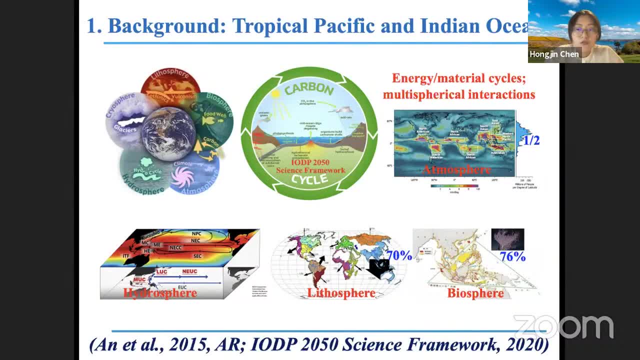 will evolve in the future. As one of the world's greatest biogeological cycles, the global carbon cycle is the key research field in the earth systems science. 2.425.35 оров- .40hc00 Daoには气体的 siblings. 데이터在地球系. Tpwa れ的地球系 底光計算器的半個人物 torn. 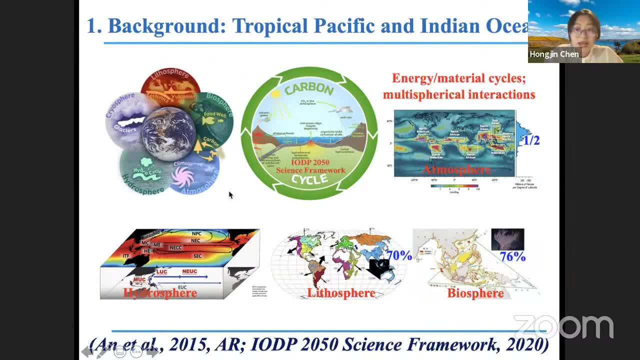 As one of the world's greatest biogeological cycles. the global carbon cycles is the key research field of the Earth system scientists integrates the multi-sphere interaction, energy and material cycle, as well as multi-discipline studies, thus attracting increasing attention from many international geoscience programs. 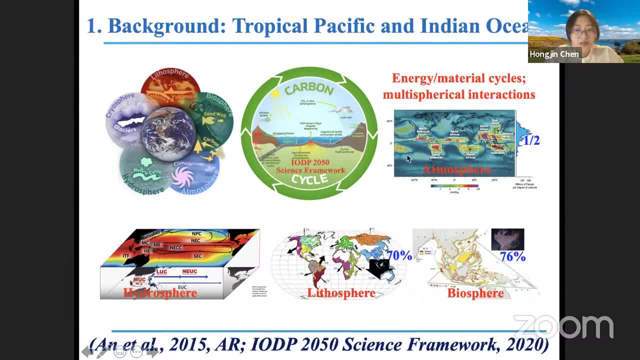 such as the IODP, The tropical Pacific and the Indian Ocean, show distinctive features in terms of different earth sphere, For example. as for the atmosphere, as one of the most intense climatic phenomena on earth, the Asian monsoon affects the leafwood of about 50% of the world's. 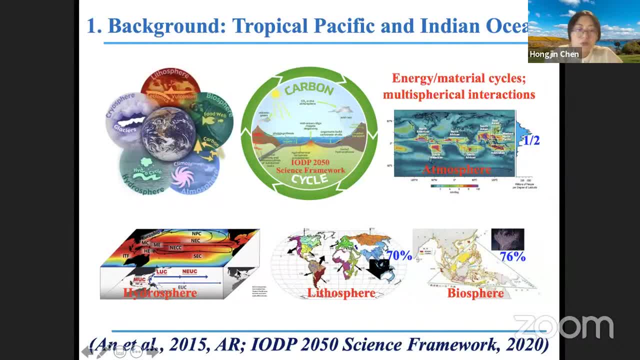 population. As for the hydrosphere, the Indo-Pacific warm pole is one of the most important components of the global ocean and climate system and acts as the major source of heat and moisture for the atmosphere, thereby driving global-scale climatic phenomena such as Erlino, southern 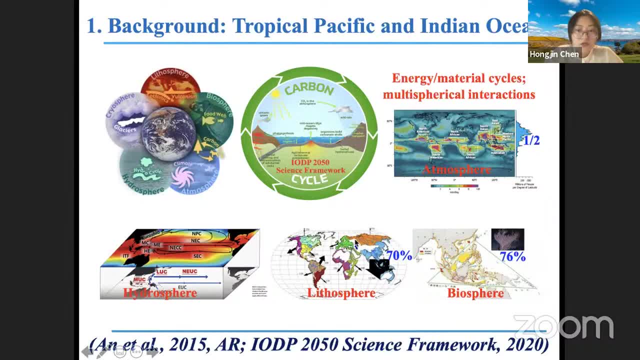 oscillation, etc. As for the lithosphere, it has been estimated that the terrestrial input from Asian rivers accounts for nearly 70% of the global fluvial sediment flux to the ocean, which makes the world's largest source-to-sink system around the continental margin. As for the biosphere, for example, 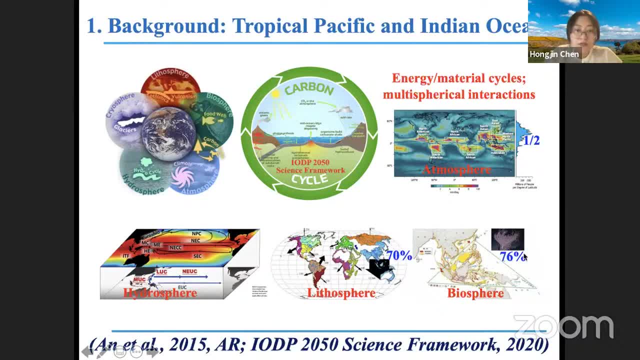 the coral triangle of Southeast Asia contains about 76% of the world's coral reef species. Therefore, the tropical Pacific and Indian Ocean constitute ideal places for the global ocean and global climate. In this way, the global ocean is a source-to-sink system. 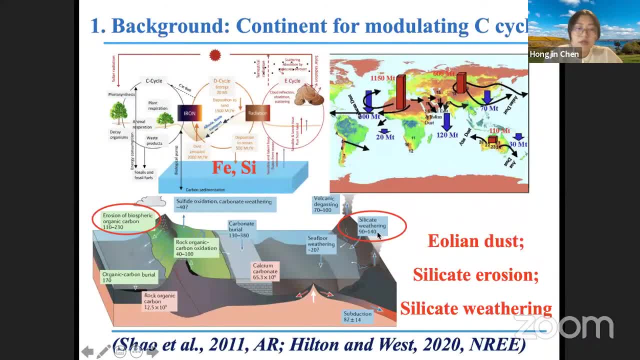 that provides the global carbon cycle. Let's now focus on the lithosphere. The Earth's surface processes, like the syndicate, weathering, erosion, together with inputs and burial of the produced detrital nutrients and organic matter to the ocean, play an important role in modulating the global carbon cycle. For 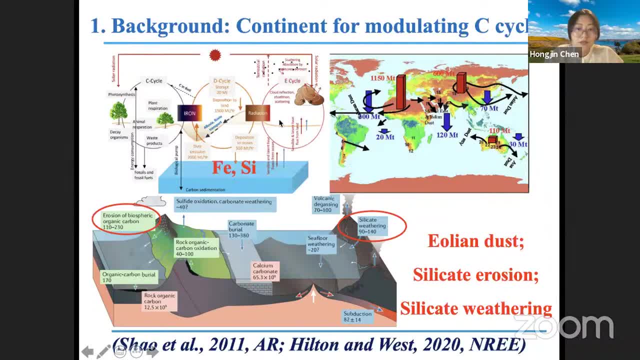 example, the Eolian dust, which is an important product of wind evolution, is a source-to-sink process for the global carbon cycle and is the most important source-to-sink process to the global carbon cycle. The Eolian dust, which is an important source-to-sink process. 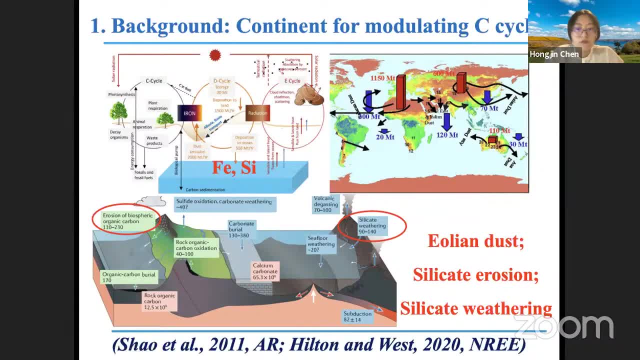 erosion on the earth's surface participates in the range of physical, chemical and biogeological process that interacts with the cycle of energy and water and carbon, And it affects the energy balance of the earth's system, carries organic matter and contribute directly to the carbon cycle, and carries iron, which is vital to ocean productivity. 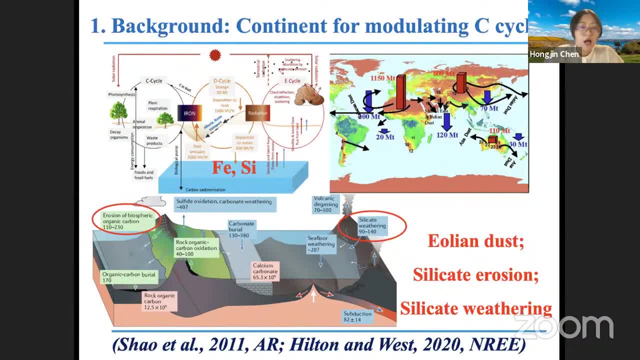 and the ocean atmosphere CO2 exchange. Besides the silicate erosion and the silicate weathering erosion, which are generally associated with monsoon precipitation, air temperature can affect the long-term ocean atmosphere budget of the carbon dioxide, both through the consumption of the carbonic acid during. 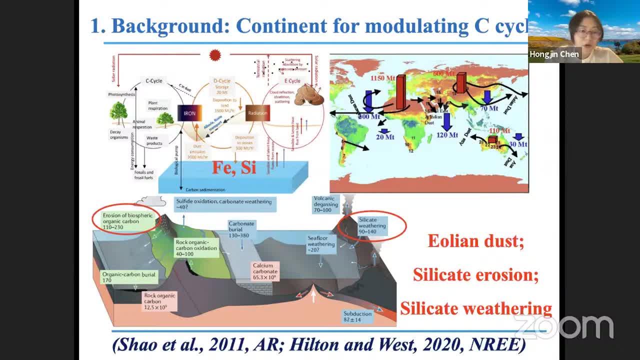 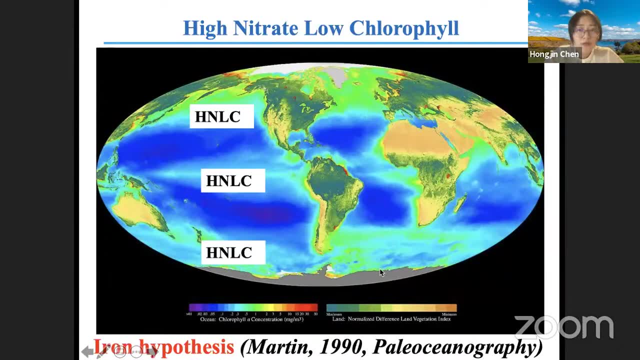 silicate weathering and through changes in the weathering and bearable rates of the organic carbon. A representative example showing the potential influence of the eolian dust to the global carbon cycle is the iron hypothesis proposed by Jean Martin. For example, the equatorial Pacific is one of the three principal high-nitrate low-chlorophyll. 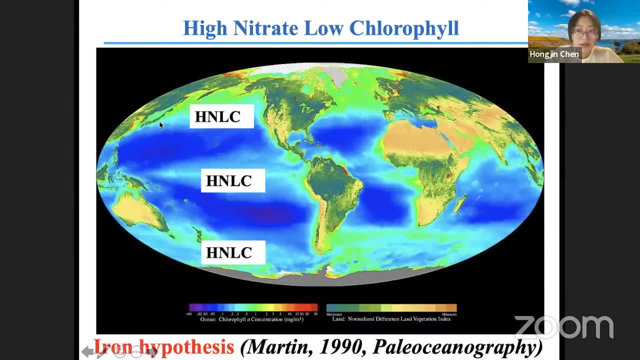 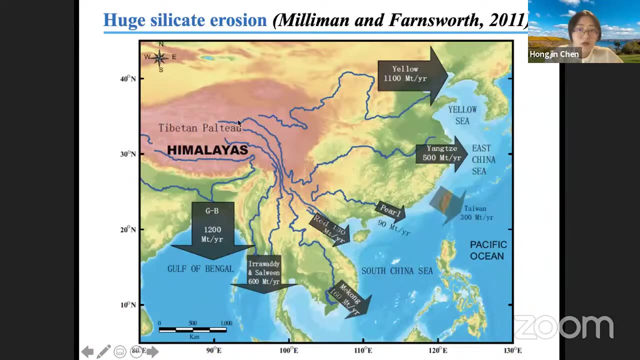 regions of the world. ocean Input of the eolian dust provides important iron supplements to the iron-limited open ocean. that stimulates primary productivity and more organic carbon burial Through the unique topography and orographic control on the Asian monsoon, the Himalaya. 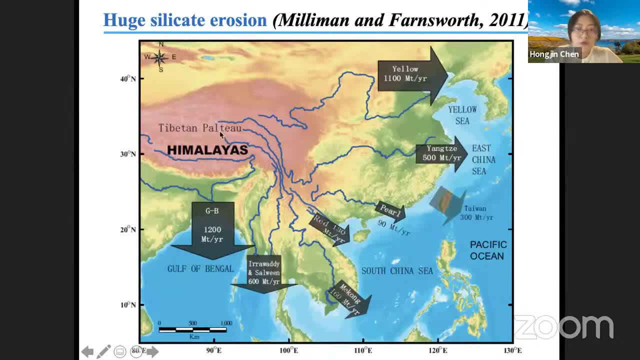 and Tibetan Plateau systems constitute the largest river erosion system of the planet. It annually carries more than a billion tons of sediments and dissolved material to the ocean, thus affecting the environment over different timescales. Currently, about 25% of the global fluvial sediment flux are discharged through the eolian. 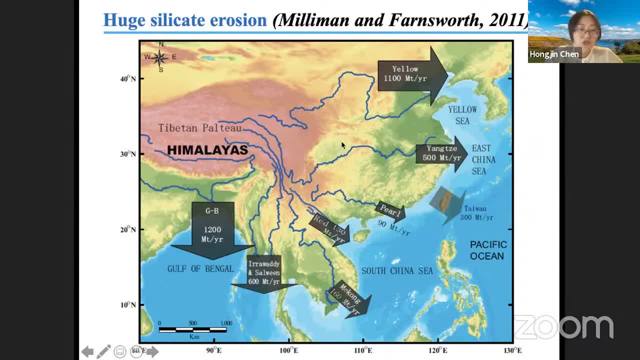 dust system. In addition, the eolian dust system has been used in several major river systems in Asia, including Yellow and Yangtze River in the East, Indus River in the West, which is not shown in this picture, and the Ganges Brahmaputra, Iwawadi, Selpham and Mekong River in the 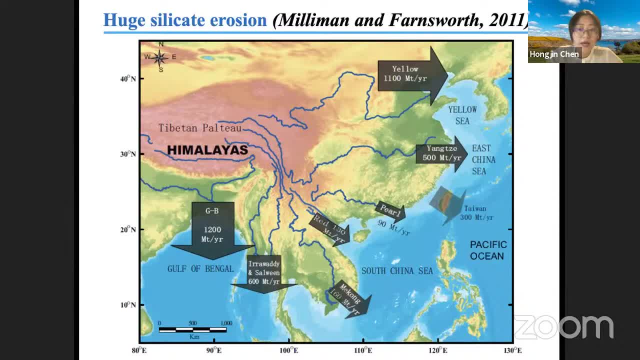 South. Among them, the Iwawadi and Selpham River annually transport 1.9 million tons of organic carbon to the ocean, suggesting that these rivers may currently be one of the largest river resources of organic carbon. In addition, the Iwawadi and Selpham River annually transport 1.9 million tons of organic 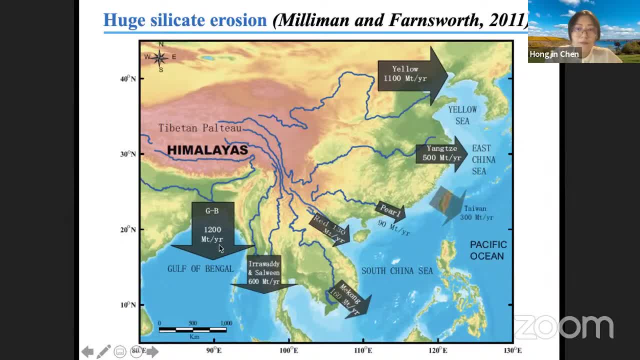 carbon to the ocean, suggesting that these rivers may currently be one of the largest river resources of organic carbon. Quantitatively, the Bengal Fan currently accounts for about 10 to 20 percent of the total торрign아s organic carbon burial in the marine sediments. 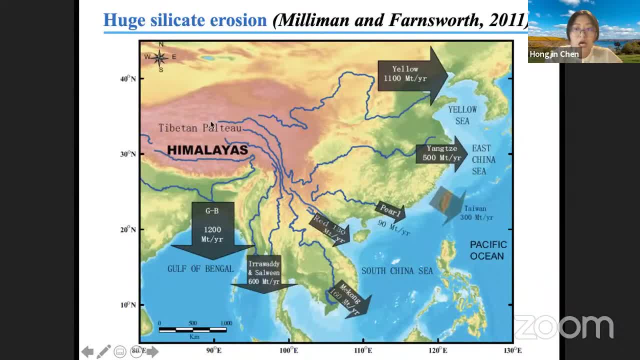 which may be more important as a mechanism for buffering the atmospheric CO2 level than the chemical weathering of the Himalayas and Tibetan Plateau. addictive during neogene or Vertetonic timescale. Next slide, please. Next slide, please. Unfortunately, the significance of the highland erosion for explaining the very large terrestrial organic carbon deposition in the eastern Arabian Sea. 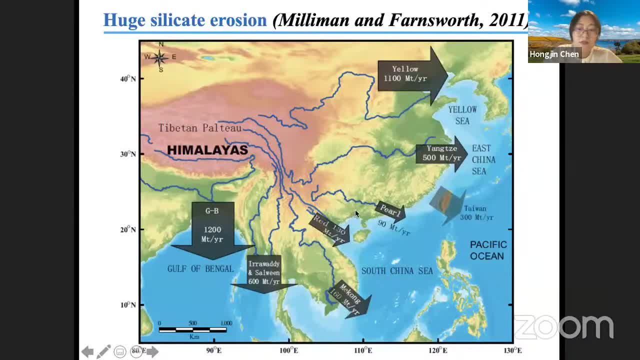 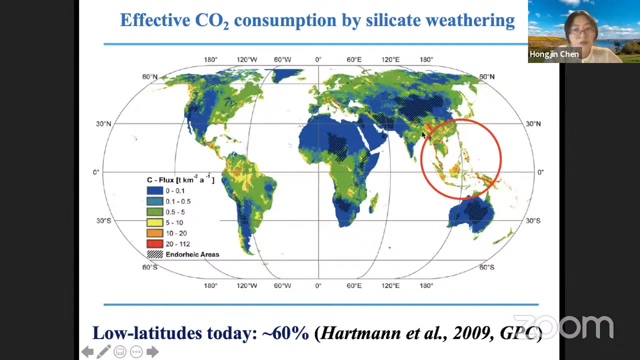 Bay of Bengal, and together with its potential contributions to the global change during the quaternary over orbital timescales, has not been quantitatively evaluated before. Besides the low-latitude Asia or Southeast Asia is a hotspot for CO2 consumption via silicate weathering. 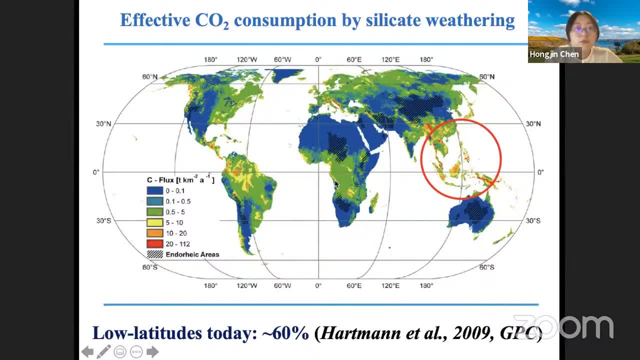 For example, this figure shows global distribution of CO2 consumption by the chemical weathering. It has been estimated that about 10% of all the atmospheric CO2 exported via silicate weathering to the ocean is persisted in about 1% of the global exorbitant. 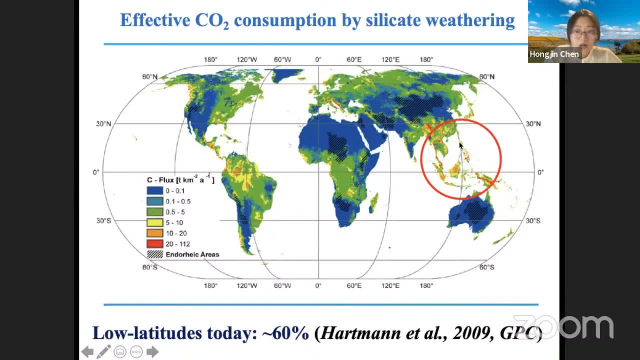 drainage area, including the volcanic arc and land like the Luzon Islands surrounding the tropical Pacific and Indian Ocean. A significant impact on the global CO2 consumption rate can be expected if these highly active weathering regions are affected by changes in the hydrological cycle due to global climate change. 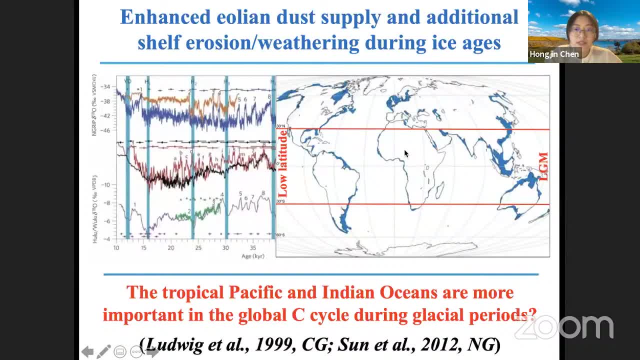 Furthermore, previous studies have suggested that the continental shelf exposed to during the LGM accounts for about 7% of the total continents of the Earth and around 48% of the new land created by the continental shelf exposure during the LGM was situated at the low latitude, which provides much wider area for silicate weathering and erosion. 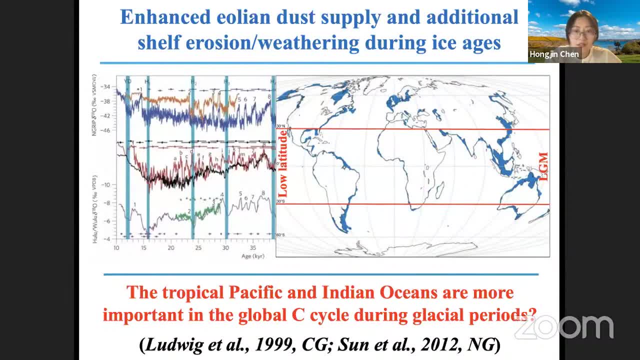 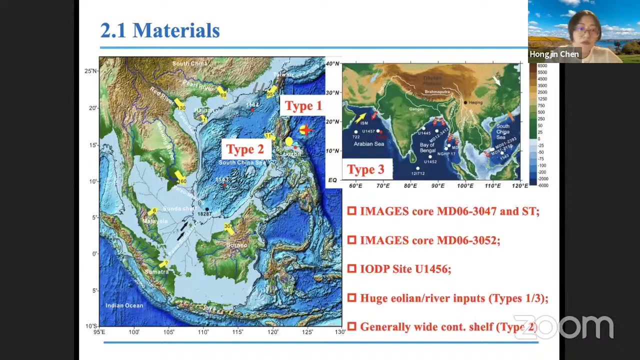 Based on the knowledge that the enhanced eolian dust supply and additional erosion weathering can be expected, the LGM is expected to be more effective in the future. In addition to the additional coastal mes alegre integrated in this study aiming to investigate the temporary and the spatial variation inter-regional, 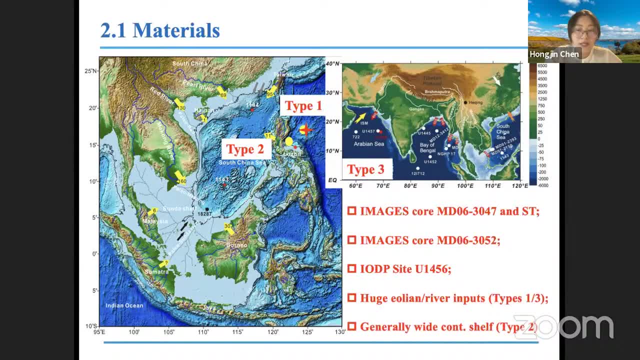 inputs of both silicy clastic matter and associated organic matter, hydrological dynamics, the panel productivity and panel redox condition and the links among these indicators, as well as the implications for the global carbon cycle. Here we divide the material that we used in this study into three types. 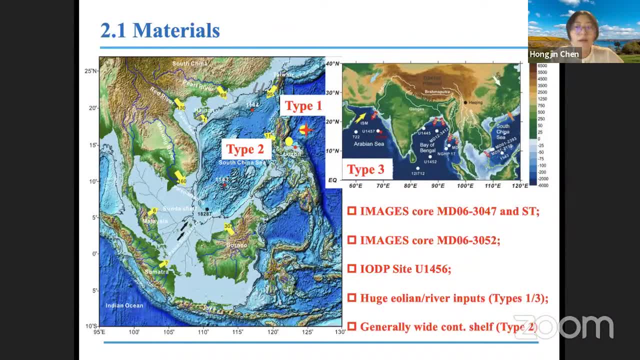 The first type includes the image core MD3047 and the modern sediment sample on the Ben Hammer rice in the Western Philippine Sea. Considering the relatively long distance between the Luzon Island and the study area, together with the relatively high topography of the Ben Hammer rice, these sediments can be used. 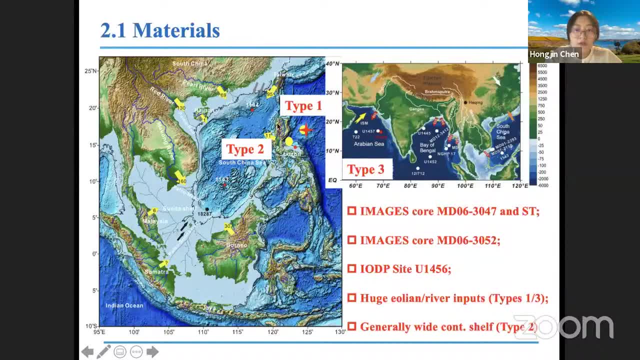 to investigate the Asian dust inputs from the mainland of Asia. Each segment represents a global carbon cycle, especially during the interglacial periods, And its implications for the East Asian winter monsoon intensity and also for the global carbon cycle, especially during the glacial periods. 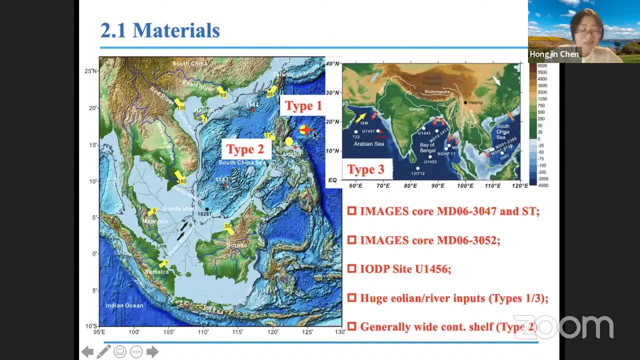 Also, this can be also used for investigate the mechanical matter supply from the Luzon Island and its implications for the East Asian summer monsoon intensity, especially during the interglacial periods. The second type refers to the image core MD03053CBr2,, which contains the material of the current 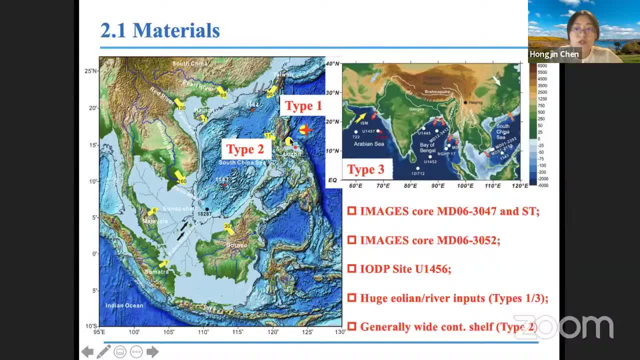 Coral ficus, which can be found within the Carpaccia climate structure, which is, in the southern quarter of Asia, Stretty. Okay, So let's start looking at the second type on the continental slope in the Western Philippine Sea. 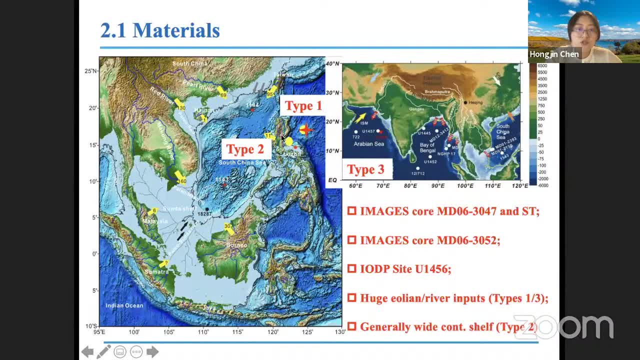 which can be used to investigate the terrestrial input from the generally wide continent around the tropical mechanic arcs like the Luzon Island in the Western Philippine Sea and its implications for the global carbon cycle during the quaternary sea level. low sands. The third type refers to the IODP site U-1456. 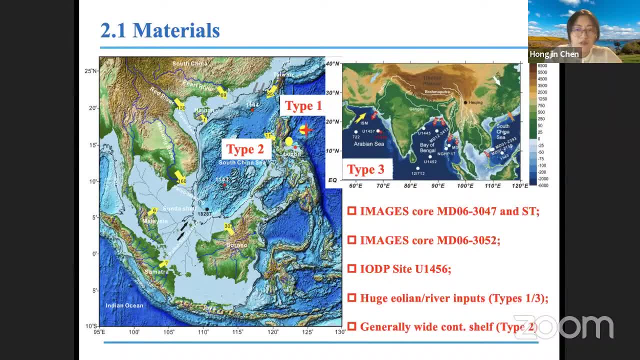 in the Eastern Arabian Sea from the Expedition 355, together with several representative reference core in the Arabian Sea, Bay of Bengal and South China Sea, which can be used to investigate the terrestrial input from the Himalaya and Tibetan Plateau and its implications for the South Asian summer monsoon intensity. 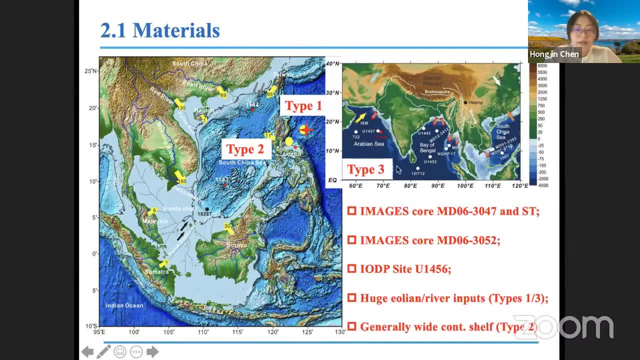 and the global carbon cycle. Here the type 1 and type 2 sediments are characterized by huge eolian dust or rivers covering sediment inputs, while the type 2 is characterized by a generally wide continental shelf. So here shows a picture of the paleogeography. 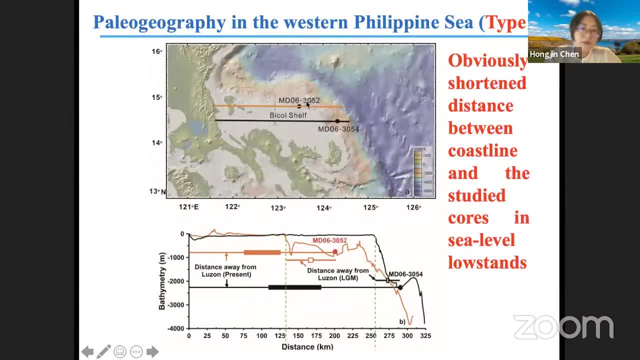 of the Western Philippine Sea and this is the sediment core MD3052 on the continental slope in the Western Philippine Sea. As you can see, during the glacial sea level low stand, the distance between the paleo coastline and the sediments is very small. 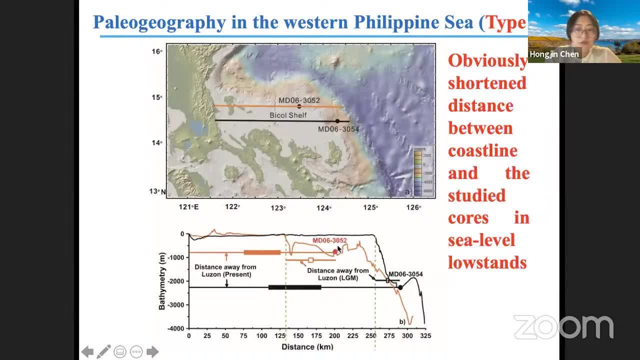 and the study core would be obviously shortened. Therefore, these core sediments preserve a paleoclimate record that serves as a highly sensitive monitor of sea level change and associated silicates, erosion and weathering of sediments on the exposed continental shelf. Here are the methods that were used. 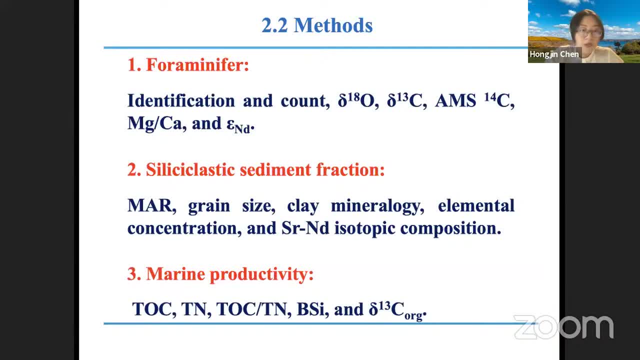 for investigating the process mentioned earlier, including the following three aspects. First, for the microfossil, we analyzed the assemblage of the four miniferal oxygen and carbon isotope and AMS, carbon-80, and elemental ratio and neodymium isotope of the forms. 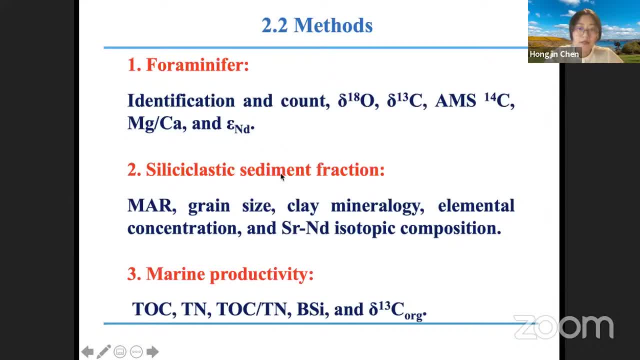 And for the SISI-class sediment fraction, we mainly focused on the mass accumulation rates, grain size, clay, mineral major and trace elements, strontium and neodymium, isotope composition, And for the box we also analyzed the organic geochemical parameters. 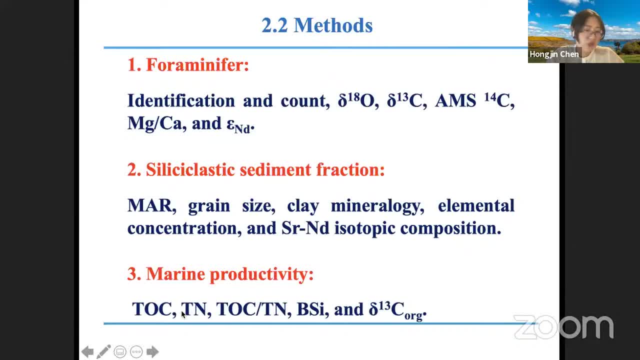 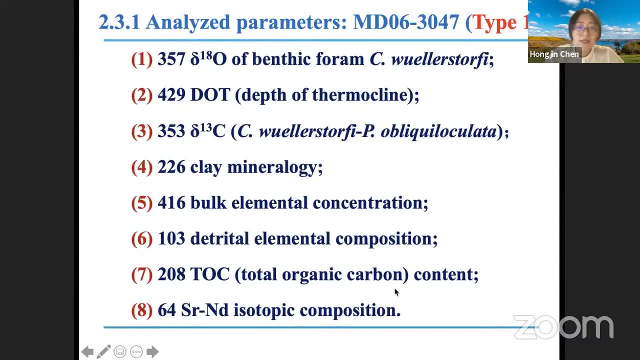 such as the total organic carbon, total nitrogen, the ratio biogenic silica and organic carbon isotopes. So in specific here I will briefly go through the analysis, the parameter used for each sediment core and to modern sediment tramp samples. 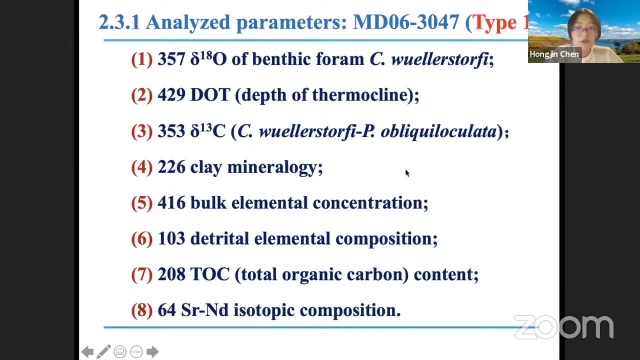 For the sediment core 3047, located on the Benham Rise in the Western Philippine Sea. we got the data set of oxygen and carbon isotopes of the forms clay, mineral major and trace elements for both bulk and the detrital fraction. 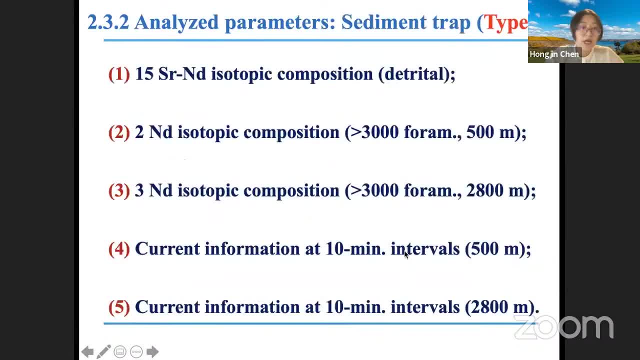 total organic carbon, strontium and neodymium isotopes For the sediment tramp sample, which covers the whole year of 2015 with 20-day interval from the Benham Rise in the Western Philippine Sea. we got the data set of strontium and neodymium isotope. 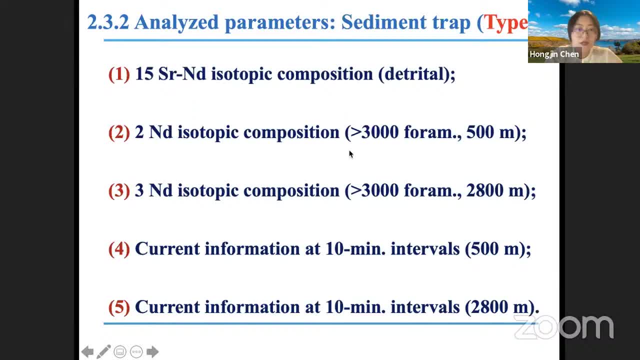 composition of the detrital fraction and neodymium isotope, composition of the planktonic for miniferal collected at a water depth of 500 meter and to 2,800 meter, And also together with the relevant high resolution current information, including the current direction. 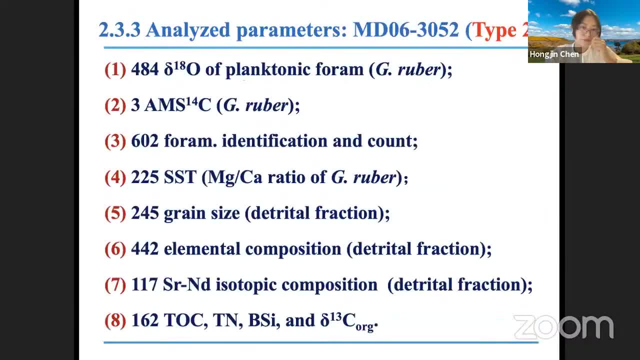 absolute speed, temperature and the simility. For sediment core MD, there are 630, 42, located on the country, the continental slope in the Western Philippine Sea. That data set actually is similar to the MD 3047. So I won't go through the details here. 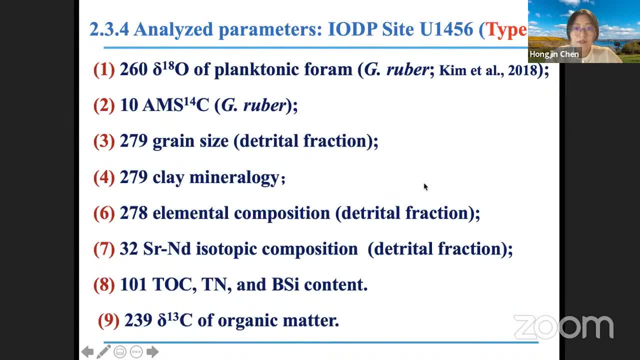 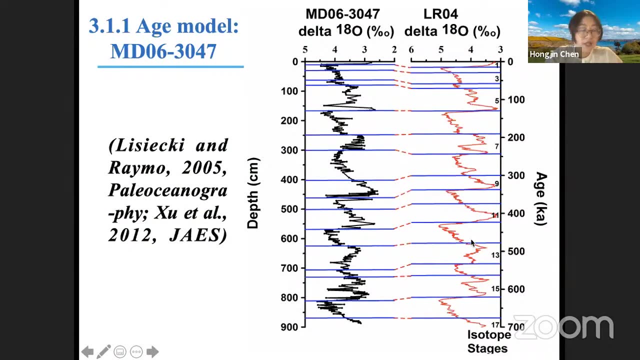 And also for the IODP site U1456 from Expedition 355, located in the Eastern Arabian Sea. we got a similar data set. Now let's take a look at the H model established for each sediment core For the MD 3047 on the Benhamma rise. 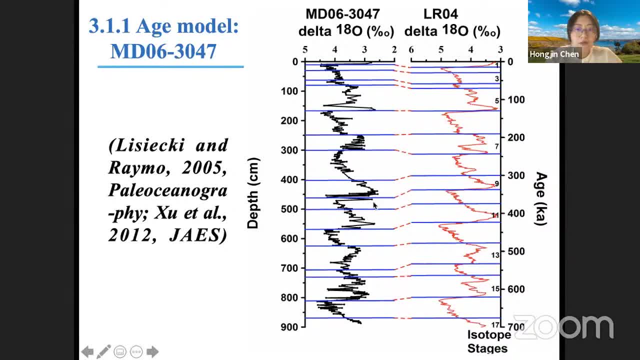 of the Western Philippine Sea. each model was obtained by comparing the oxygen isotope curve for the benthic for miniferal with the standard LR04 stack. As a result, the study course spans MI as one to 17.. That's recording the panel environmental history. 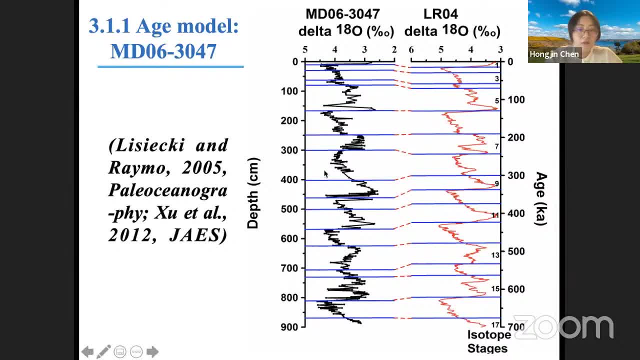 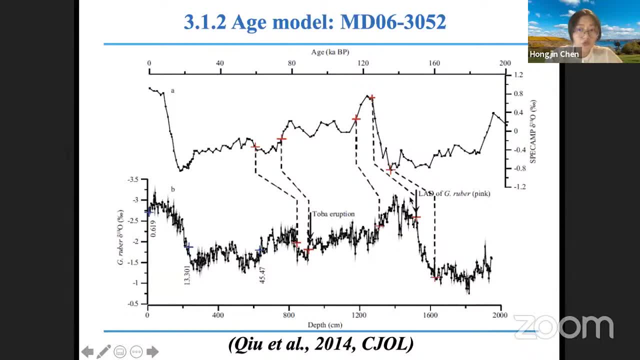 of the last 700,000 years, with sample solution of about 3,000 years For sediment core 3052 from the continental slope in the Western Philippine Sea. Similarly, the H model was reconstructed based on the correlation of the planktonic forums oxygen isotope data. 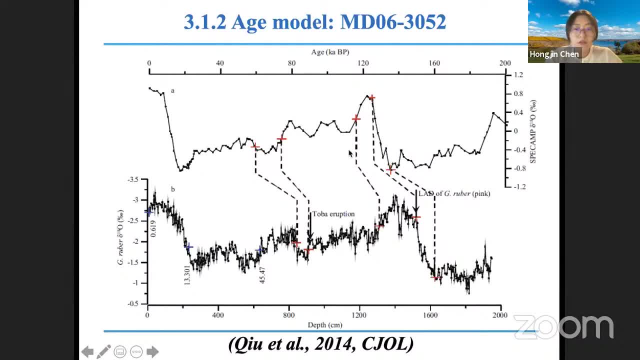 to the standard oxygen curves, combined with three AMS carbon dating from the past 45,000 years. As a result, this core is known to span MI as one to six, thus potentially recording the panel, but it's still a little bit of a long way to go. 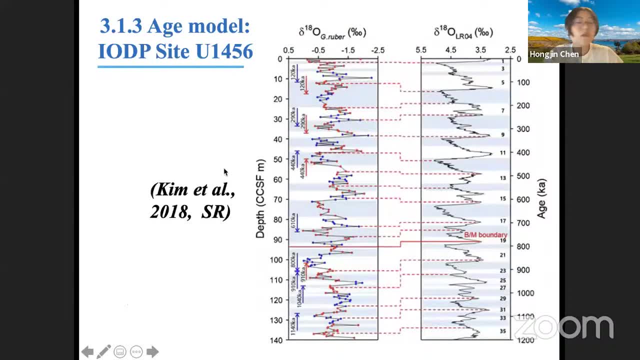 Now let's take a look at the H model for each sediment core For the MD 3047 on the Benhamma rise of the Western Philippine Sea. each model was obtained by comparing the oxygen isotope curve for the benthic for miniferal 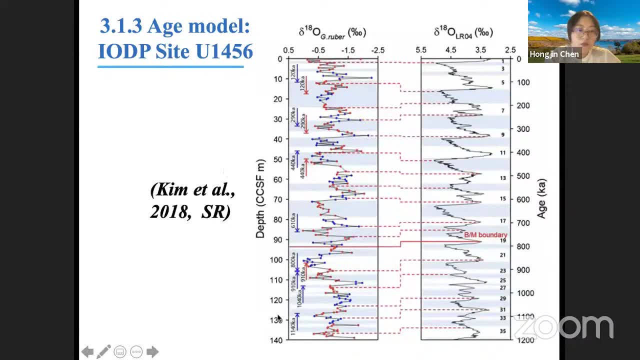 with the standard LR04 stack. As a result, the study course spans MI as one to 17.. That's recording the panel environmental history since 156,000 years. For the IODP site U4056,, we mainly focused on the upper 140 meters of the core. 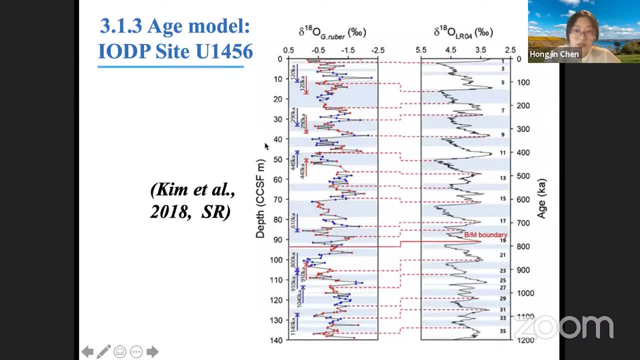 Similarly, the H model of the investigated intervals was mainly established by correlating the planktonic for miniferal oxygen isotope record to the LR04 benthic oxygen isotope stacks. So the H model combined with onboard biostratigraphic 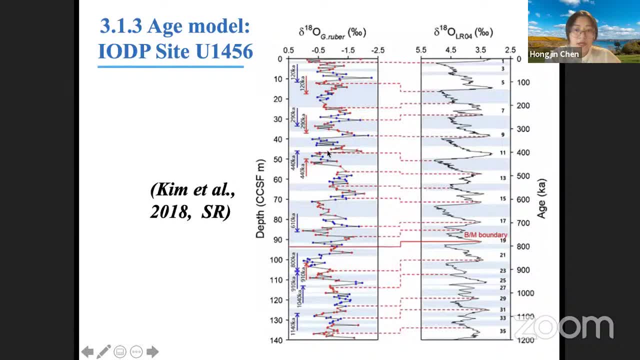 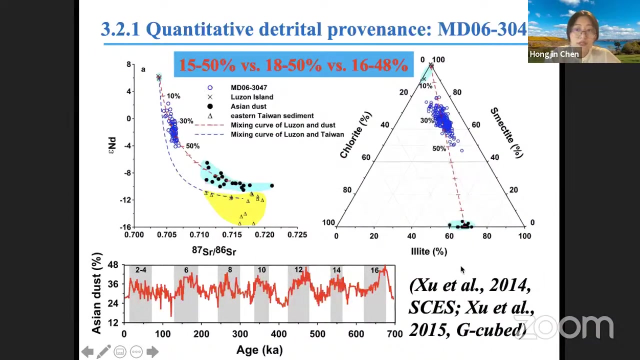 and panel magnetic records, And this correlation indicates that the upper 140 meter section spans MI as one to 35, thus covering the past about 1.2 million years, with an average sampling resolution of about 4.2 million years. Now let's move on to the quantitative detrital sediment. 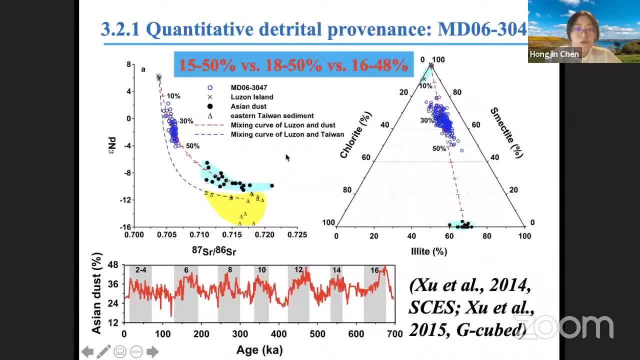 provenance distribution. First, the sediment core MD 063047 on the Benhama Rites of the Western Philippine Sea Here shows two figures of discrimination: plot of strong-shell and neodymium isotope and the clay mineral assemblages of the study site and the potential sources which mainly 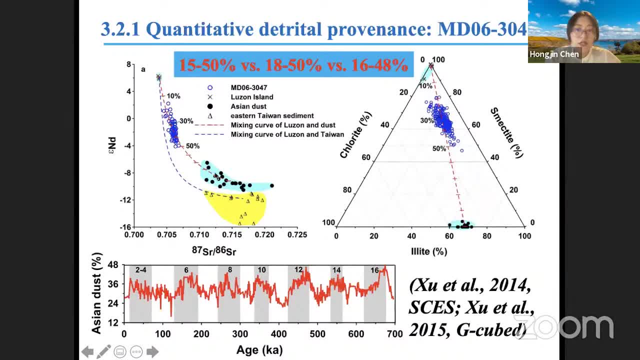 includes the Luzon Island, the Eolian Dust from Asia and fluvia sediments from East Taiwan. Down here this figure shows the temporary variation of Eolian Dust input to the study site, calculated by the discrimination function based on the rare earth element. 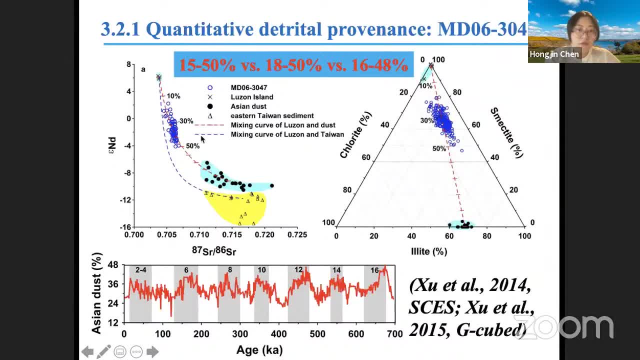 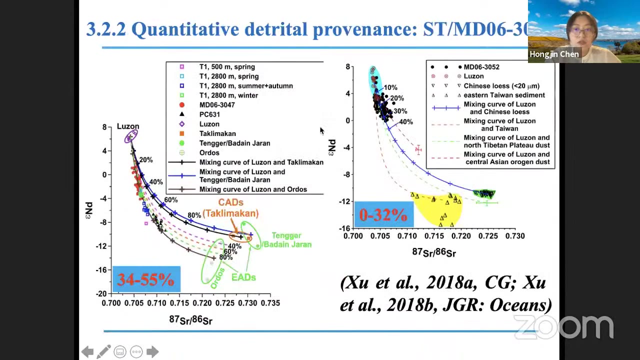 These three different plots consistently indicate that the remote Asian dust and the nearby Luzon volcanic arc matter are the primary detrital sources, in which the contribution from the Eolian Dust accounts for about 15% of the Eolian Dust, And the second for the modern sediment tramp and sediment core MD 3052 in the Western Philippine. 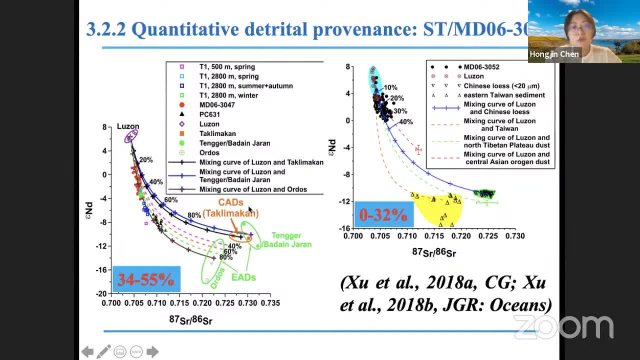 Sea. Here are the two discrimination plots showing the composition of strong-shell and neodymium isotope of the detrital fraction sediments in the study sample and the potential sources respectively. The left one shows the comparison of the modern sediment tramp and sediment core MD 3052 in. 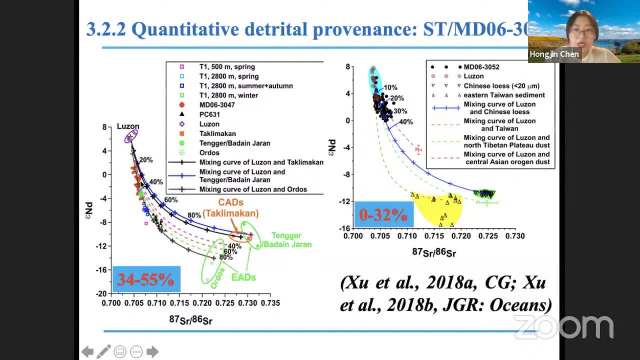 the Western Philippine Sea. Here are the two discrimination plots showing the composition of strong-shell and neodymium isotope of the detrital fraction sediments in the study sample and the potential sources respectively. The right one is the comparison of the information for antimon 문 solid mud litter patterns. 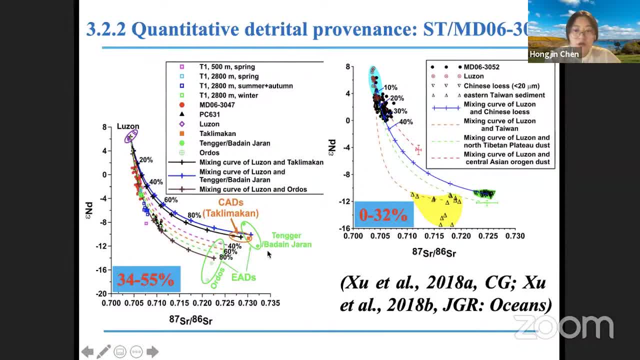 using the standard alpha test, the traditional method of collecting preferred conditions. Pedestrian Ed Thompson, луч 205. Not a video. So, again, as I said, such auş ayudar to access this piece lower. this is the improvement based on this particular experiment. 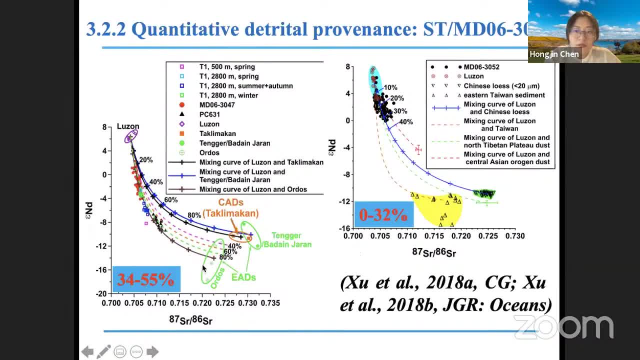 The negativeник is derived mainly from the Eastern Asian deserts or all those deserts, and to a lesser extent from the Taklamakan, Bandajere and Tango deserts. The right one shows the combination of the sediment core 3052 and the similar potential sources. 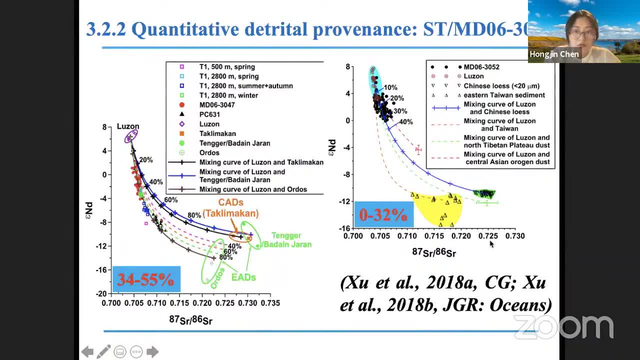 including the volcanic rocks from the Luzon and East Taiwan sediments, as well as the fine-grained Chinese Luz Quantitative calculation based on the strontium and the neodymium isotope, indicate that detrital fraction of the sediment core were mainly sourced from the Luzon. 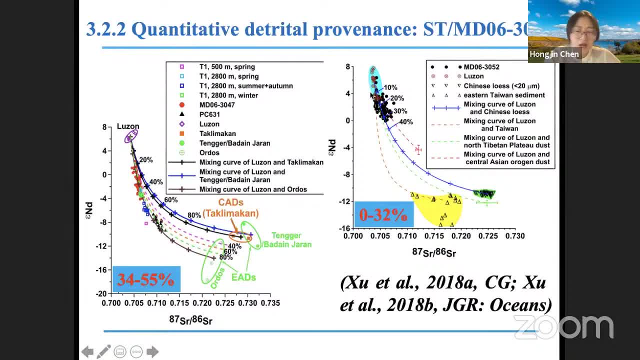 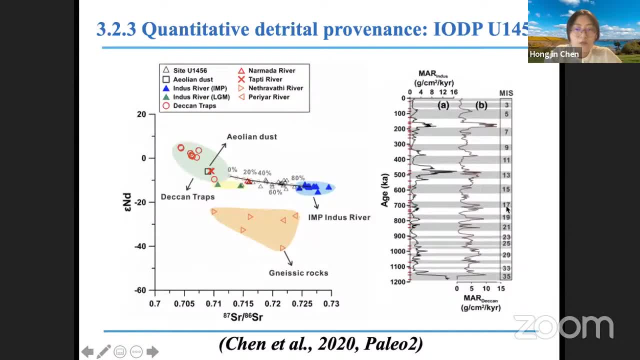 which accounts for 68 to 100% and to a lesser extent from the Asian continent. The isotope strontium and neodymium composition are also used to identify the detrital provenance of IODP sites U-4856 in the Eastern Arabian Sea. 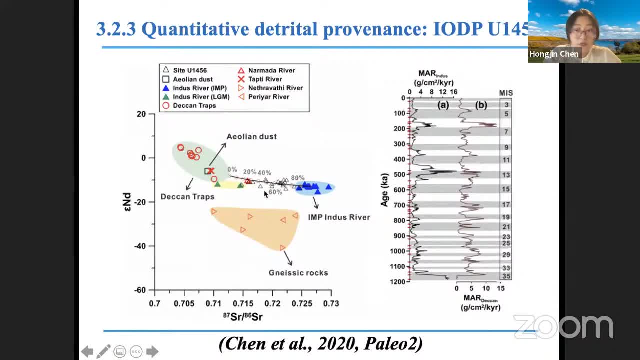 By comparing to the signatures of the potential sources, which includes the Indus River, Deakin Tramps and the nice thick rocks from the South India and the Aeolian dust, we conclude that the clay-sized detrital sediments of the study site were mainly derived. 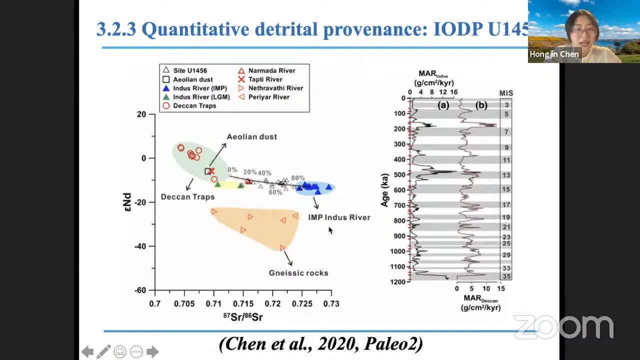 from the Indus River and the Deakin Tramps. Besides, the temporary variation of the mass accumulation rate of different sources suggests a abrupt increase in the terigenous input from the Indus River during MIS-12 to 13,, which may have resulted from intensive physical erosion. 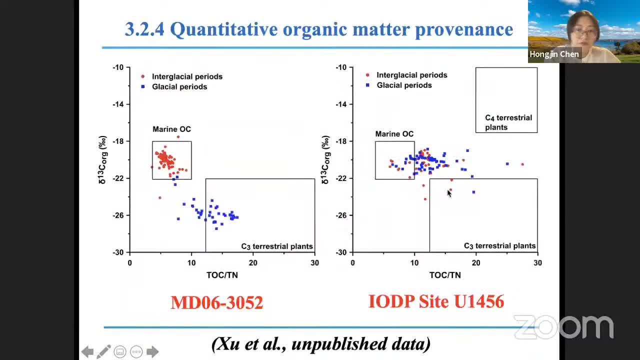 events in the Himalaya and the Tibetan Plateau region. Besides, we also analyzed the sources of organic matter for the core MD-3052 and the IODP sites, Using this discrepancy plots of organic carbon isotope, the ratio of total organic carbon to the total nitrogen. 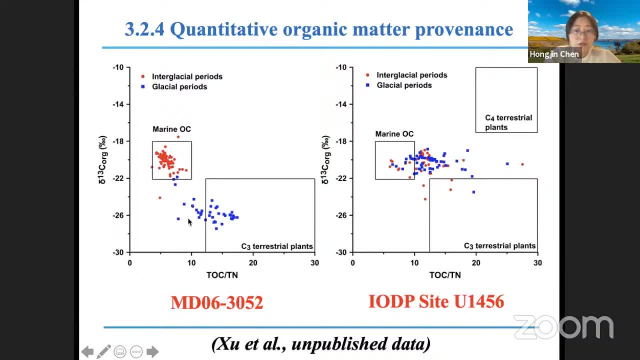 As we can see from this left plot, organic matter in the core MD-3052 show clearly different sources during the glacial and interglacial periods, indicating the enhanced barrier of terigenous organic matter during the glacial periods. In addition, as shown in the right plot, 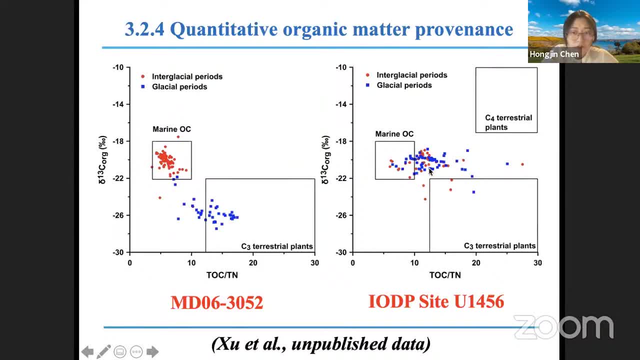 organic matter at the IODP site U-4056 derived from the MIS-12 from both marine source and terrestrial sources, And the terrestrial sources can be further divided into two types- C3 plants and C4 plants- And over time scales it is actually characterized. 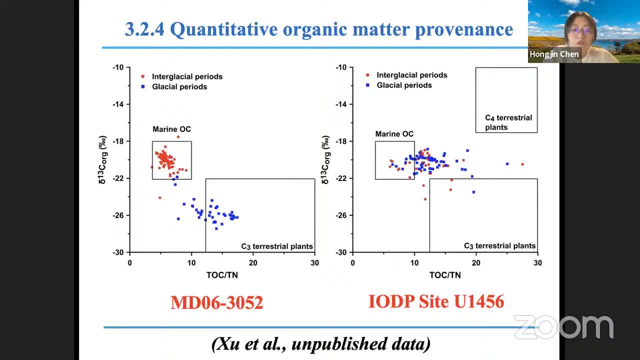 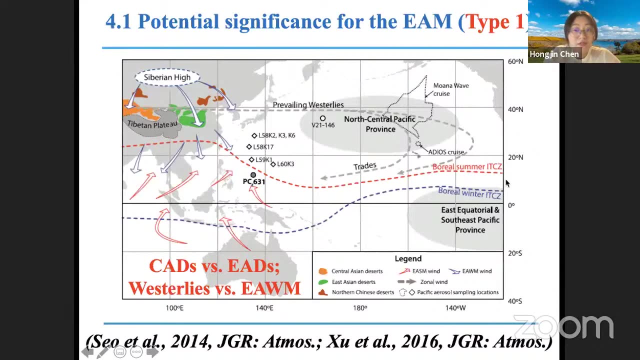 by a slight increase in the mass accumulation rate of organic matter for both marine sources and the terrestrial sources during the glacial periods relatively to those during the interglacial periods, Based on the quantitative sediment provenance discrimination results. now let's take a look at the potential significance. 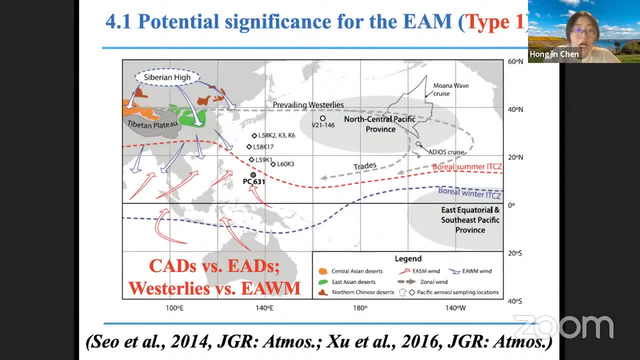 for the variation in the East Asian monsoon intensity. The tropical and subtropical Northwest Pacific is influenced by the seasonal reversal of prevailing surface winds due to the East Asian monsoon system and the associated movements of the ITCD. It is generally accepted that the westerlies 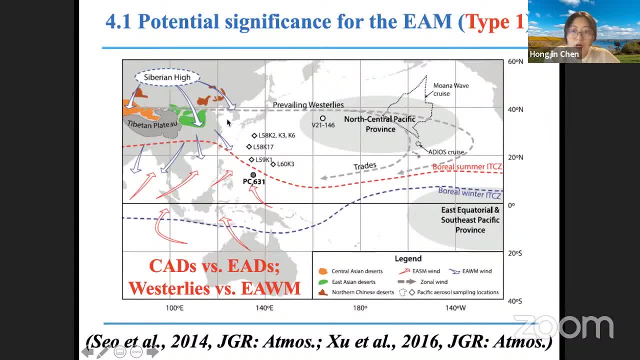 and the East Asian winter monsoon are the major driver of the Yolin dust from the mainland Asia to the Pacific, And the dust can be transported to the West Pacific from various sources, such as the West Asian deserts and the Central Asian deserts, by the East Asian winter monsoon. 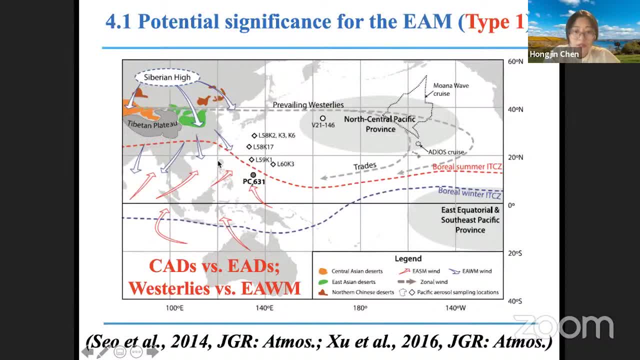 or the westerlies volcano islands in the Western Pacific or from the Australia deserts. Actually, the Central Asian deserts and the Eastern Asian deserts are the most important Asian dust sources, although their respective fluxes are not always easy to resolve. 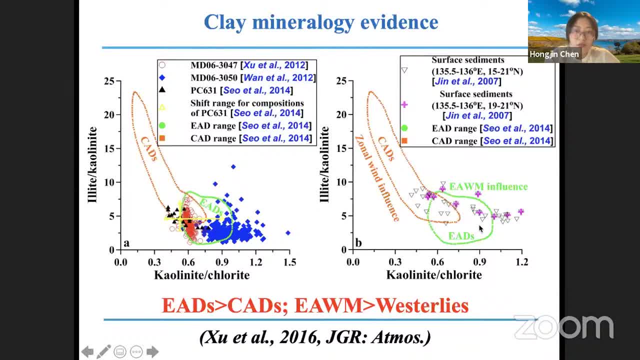 Here, by using the discrimination plots of the clay mineral ratio- elite versus collinite, collinite versus chloride- we can discriminate its actual sources. The clay mineral data from the sediment core 3047 from the Western Philippine Sea are most similar to the Eastern Asian deserts. 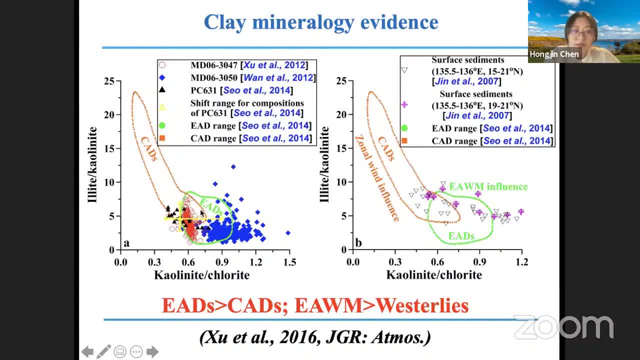 which is shown by this green ellipse here instead of the Central Asian deserts. Besides, it's also supported by the surface sediments collected from the Northern Central Philippine Sea, which also show affinity with the East Asian deserts. So altogether, such observations suggest that 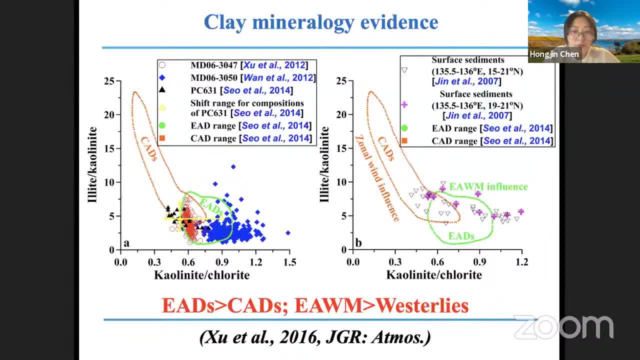 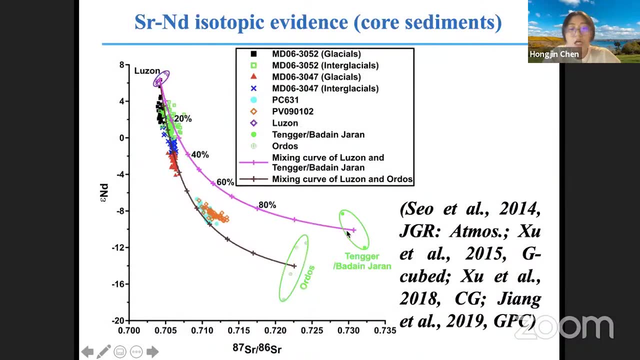 the Yolin dust deposited in the Western Philippine Sea during the middle-late quaternary appears to be mainly sourced from the Eastern Asian deserts via the north-westerly surface winds associated with the East Asian winter monsoon. Besides, the conclusion can be also supported. 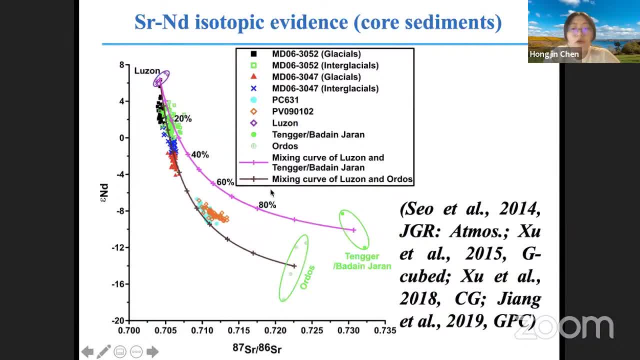 by the strontium and neodymium isotope from the sediment core in both the Western Philippine Sea and the Eastern Philippine Sea, which further suggests that significant contribution from the East Asian deserts, such as the Odos deserts, Tengor and Banjiri deserts. 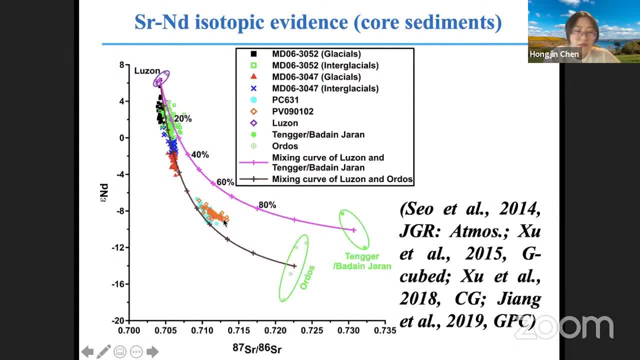 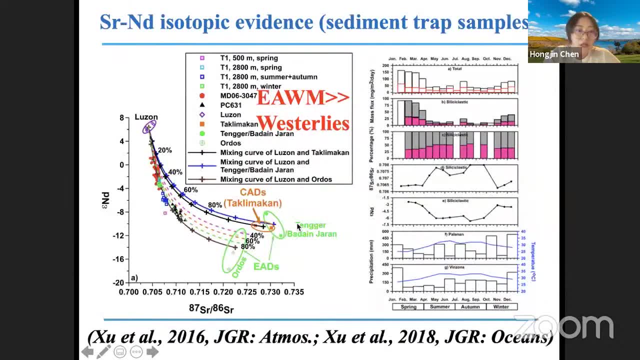 to the sediment core- MD 06-3047,- especially during the glacial periods. As for the modern times, strontium and neodymium isotope evidence from the sediment tram sample also indicate that the modern Eolian dust transported to the Benhamma rise. 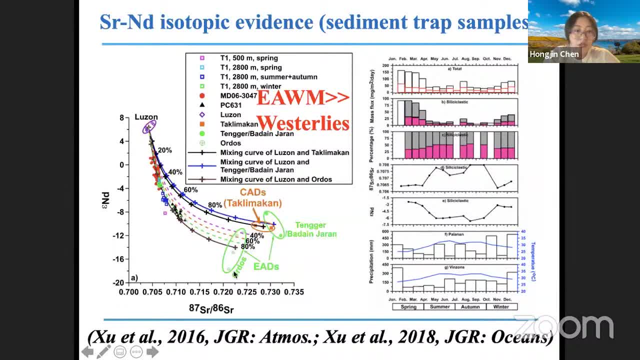 is derived mainly from the East Asian deserts, which accounts for over 80% of the sediment, And to a lesser extent from the Taklamakan, Benajiri and the Tengor deserts, Besides the fluxes of both dual-zone volcanic matter. 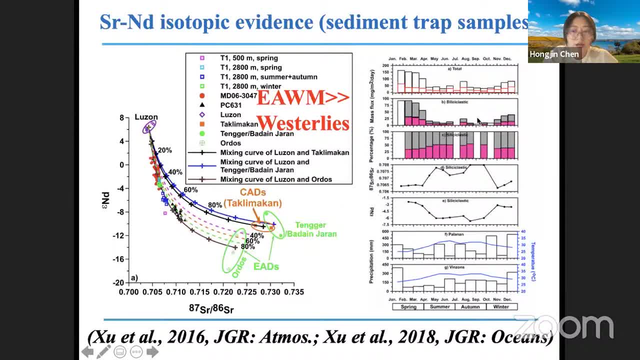 and Eolian particulates are characterized by seasonal variability. The highest of value occurs in spring, followed by in winter and then summer and autumn of the year 2015.. The East Asian precipitation and the East Asian winter monsoon density are the dominant factors in the data. The standard ofcken-roman analysis for the West Asian desert, which is based on the Tengor desert. the bind and tangerine has been conducted on both the C-A1-E operatic and Tengor desert, as well as the Tengor desert. So we can see that the the National Geographic has veneration on both the East Asian deserts. 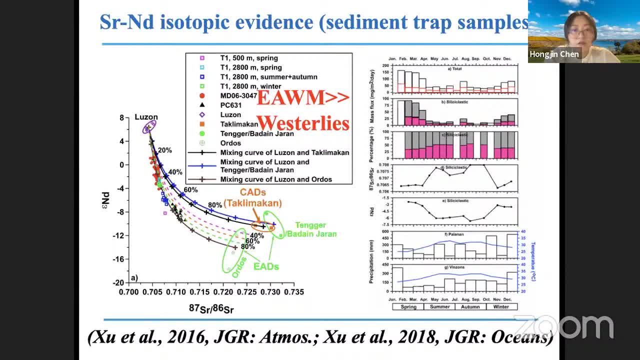 the dominant controlling factor on the changes of these mass fluxes. So, in summary, we conclude that the East Asian winter monsoon and East Asian summer monsoon are the most important transporter for the East Asian deserts and the Luzon volcanic matter deposited in the Western Philippine Sea. 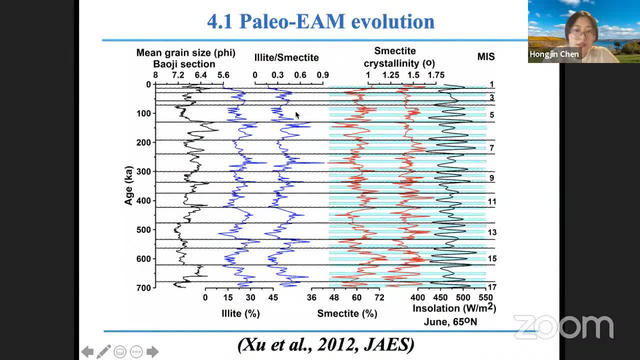 Based on the above conclusion here, as e-light is primarily derived from Asian continent and continent with eolin origin, while smactite originates predominantly from the alliteration of the nearby Luzon volcanic rocks. Here the e-light versus smactite ratio at the sediment. 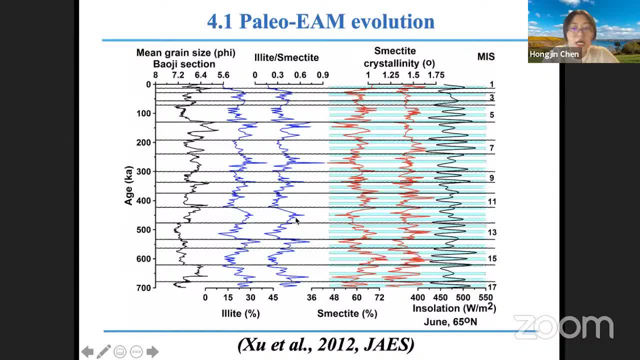 core MD3047 can be used to trace the East Asian winter monsoon variability, while the smactite content and smactite crystal nility can be used to constrain the East Asian summer monsoon evolution. As we can see in this figure the downfall. 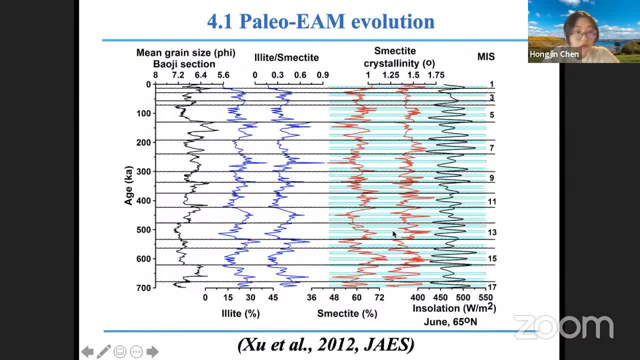 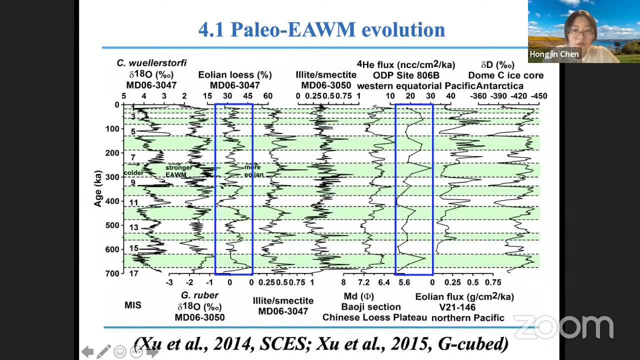 core variation of the clay mineral-related parameter all show clear glacial and interglacial cycles since the last 700,000 years. Besides the quantitative estimation of the eolian dust content of this sediment core, as shown in this left blue box here which 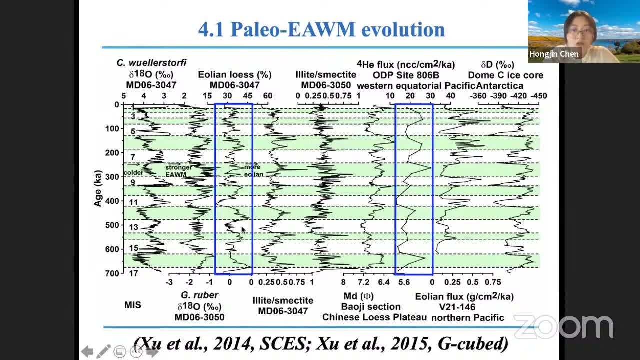 was calculated based on the 2N member mixing model, can be also used to reconstruct the evolution of the East Asian winter monsoon Over orbital timescale. evolution dust content display. the similar temporary variation with the 4-helium-based eolian import record. 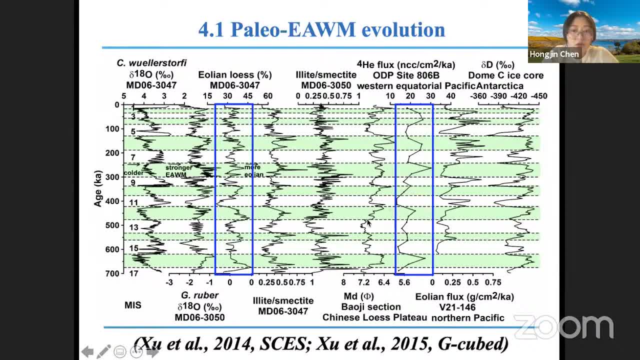 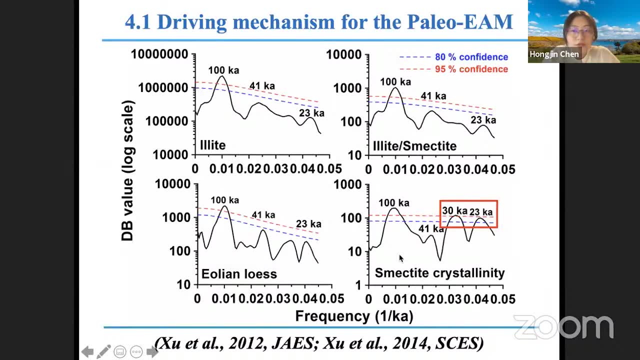 at the ODP site in the Western Equatorial Pacific, as well as the medium grain size from the Chinese Lust Plateau, which show clear glacial interglacial cycles with strong East Asian winter monsoon during the glacial periods. Furthermore, Spectral analysis were performed. 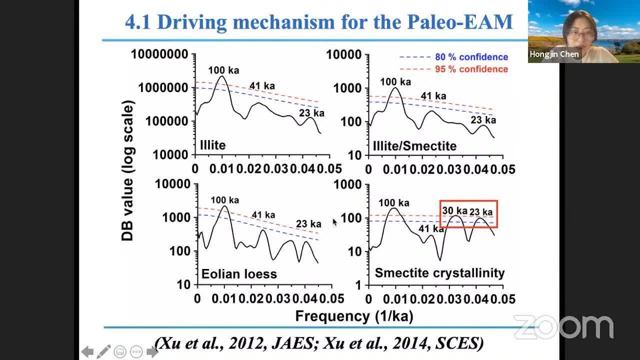 in four typical parameters related to the intensity of the East Asian monsoon. As you can see, the power density spectrum for all parameters show an obvious 100,000-year cycle above the confidence level of 80% to 95% which is attributed to the orbital eccentricity. 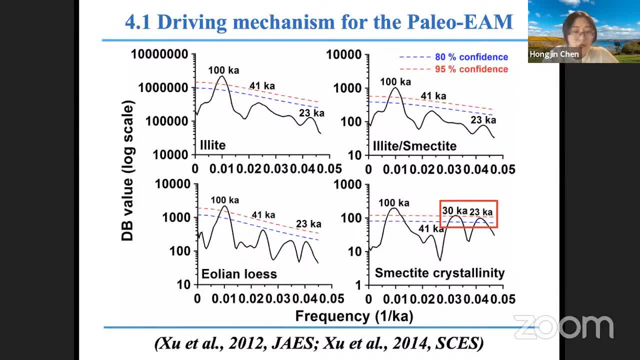 This 100,000-periodicity of the orbital eccentricity which is commonly related to the late quaternary glacial and interglacial oscillation seem to be the most important control mechanism for driving the clay mineral input in the Western Philippine Sea during the last 700,000 years. 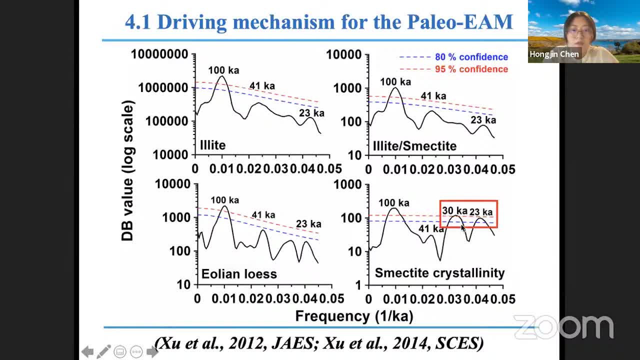 Besides, it should be noted that the downcore variation of the smactite crystallinity value shows strong periodicity of the 30,000-year cycle and 23,000-year cycle. This 23,000-year precession cycle is a major component. 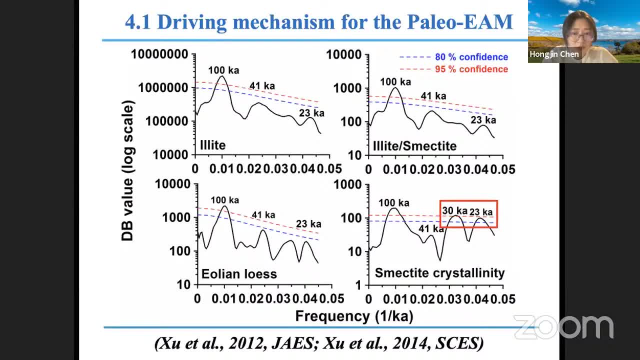 in the low latitude summer insulation variability which is commonly identified in the Eastern Asian summer monsoon proxy. As for the strong 30,000-year cycle, it is commonly attributed to the hetero-dye frequency of the primary orbital period and has been interpreted to reflect. 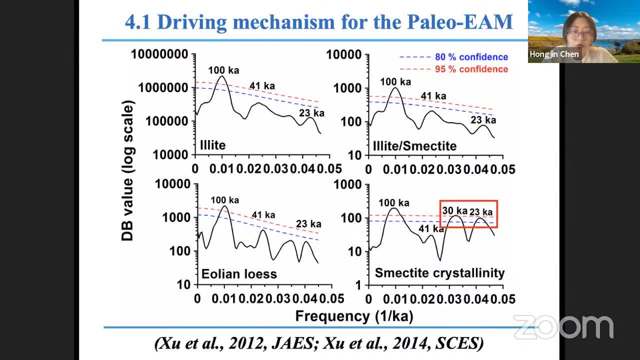 the nonlinear driving process which appears in the two-year cycle. In addition to this, it is also a major factor in the long-term and interglacial cycle of the East Asian summer monsoon. This has been interpreted to reflect the influence of the long-term and unsoil-like forcing. 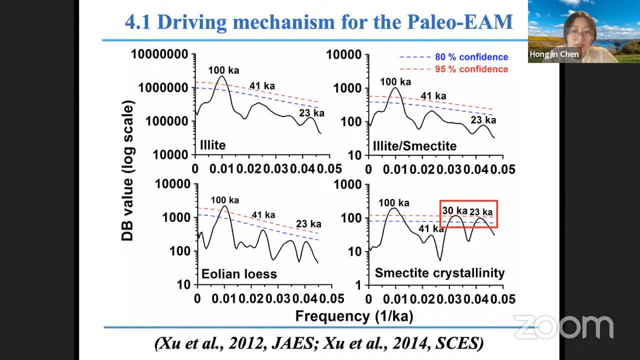 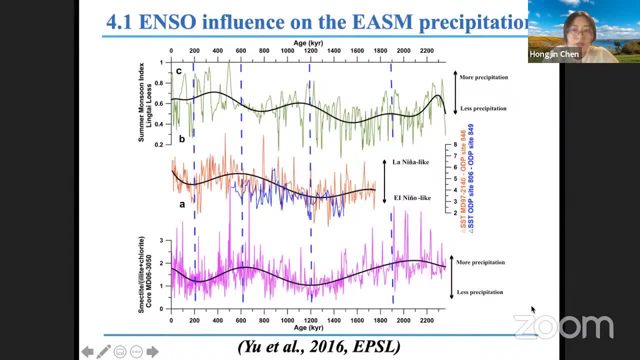 like anti-glacial and interglacial cycle in the East Asian summer monsoon. Actually, the unsoil influence on the East Asian summer monsoon precipitation has been further evidenced by another sediment core also on the Benhamma rise in the West Asian summer monsoon. 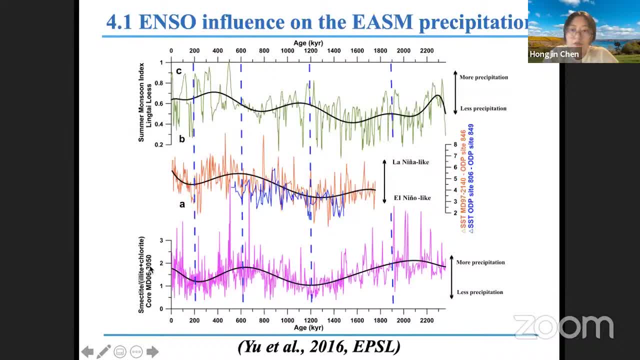 This is the sediment core MD 3050. over a longer time scale. This study showed a temporary variation in spatial co-evolution of the monsoon precipitation, as evidenced by the ratio of smactite versus elite plus chlorides, and to the tropical Pacific anisotropic system. 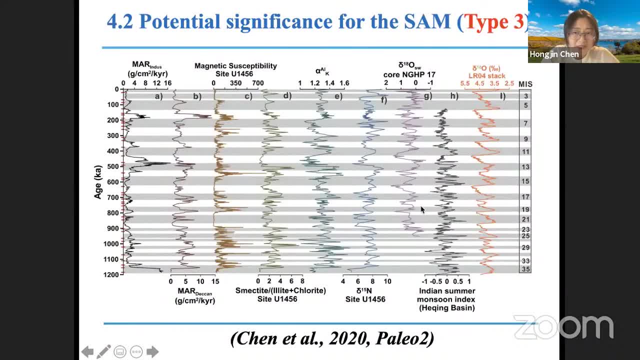 In the case of IODP site U1456 in the Eastern Arabian Sea, its sediment record is higher than the US, so it is highly controlled by the South Asian summer monsoon system. Here the ratio of smactite versus elite plus chlorite: 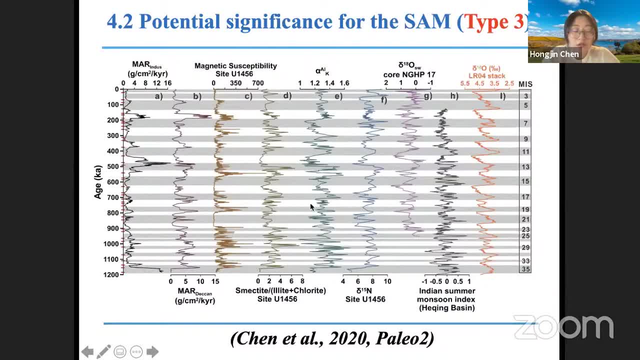 and the ratio of aluminum versus potassium, which are closely related to the syndicate chemical weathering intensity in the source regions, were used to reconstruct the South Asian summer monsoon intensity During the most interglacial and even certain glacial periods. the South Asian summer monsoon- patienceaben. 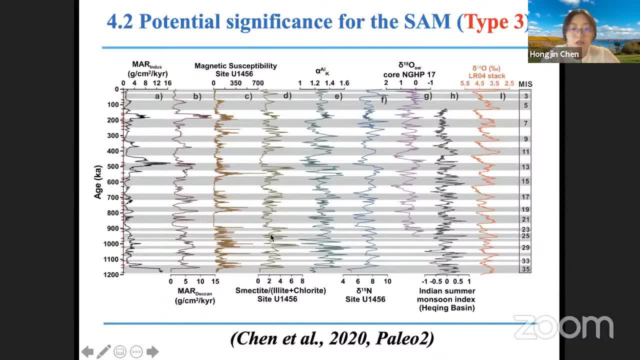 reinforcement is closely coupled with enhanced continental chemical weathering and physical erosion. Besides, we also observe a significant fluctuation in syndicate weathering and erosion during the interval of 1.2 to 0.7 million years, which indicates an enforcement of the 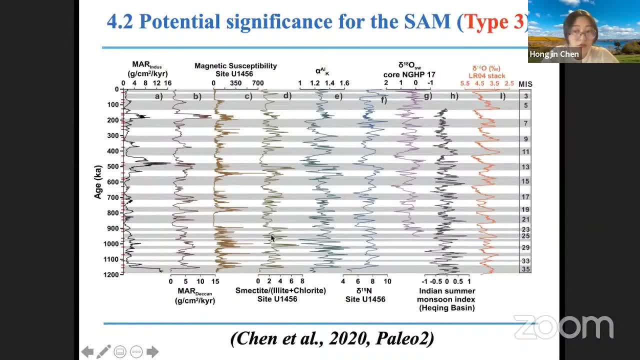 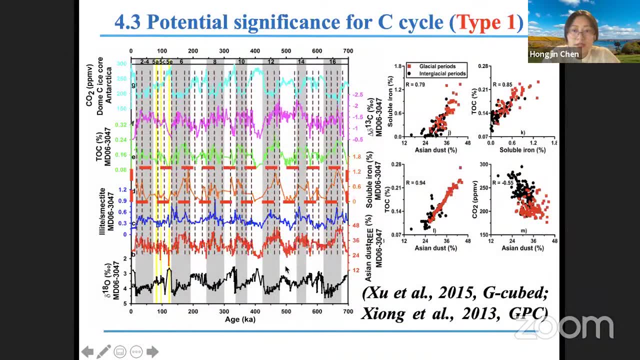 South Asian summer monsoon, with increased variability in association with the middle Pleistocene transition. So now let's take a look at the potential significance for the global carbon cycle For the first type of scenario, like the sediment core on the Benama rise in the Western Philippine. 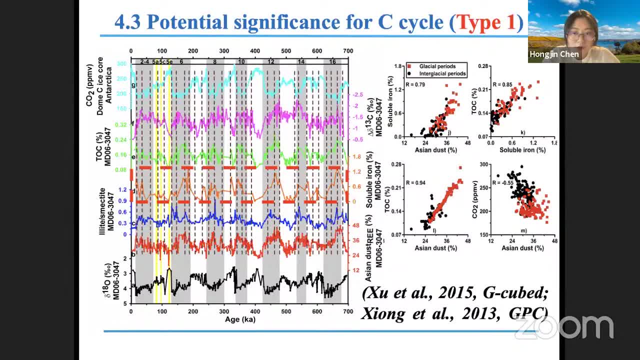 Sea, which is far away from the continent, like the Philippine island, and prevented from direct terrestrial input by the deep trench. the input of Eolian dust and its consequent process may play important role in modulating the carbon dioxide during the glacial intervals. 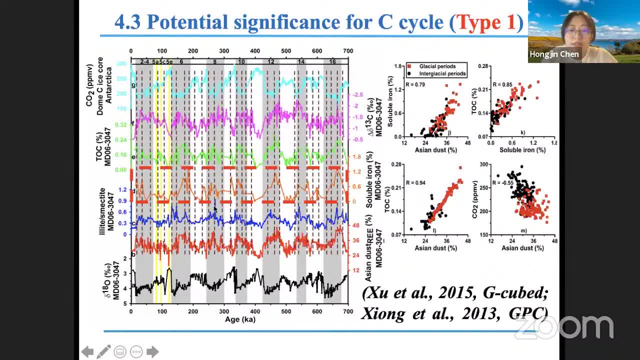 As shown here, combined with selected proxy overglacial and interglacial timescales, enhanced Eolian dust input was recorded in the sediment core 34.7 during the glacial periods, thus stimulating the biological productivity as evidenced by the difference between the carbon. 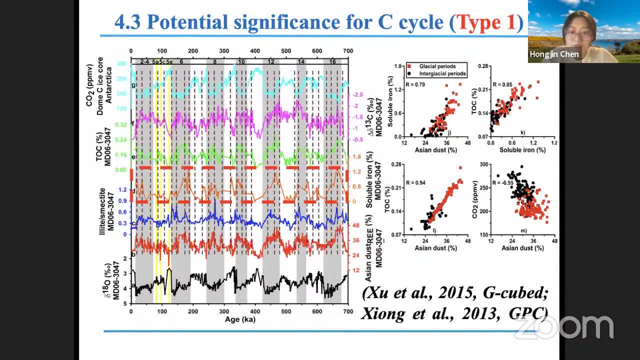 carbon isotope of the benthic and planktonic foraminifera and also the barrier of large amounts of organic carbon and dust. contribution to the reduction of the atmospheric carbon dioxide concentration during the glacial periods. This hypothesis can be further supported by the 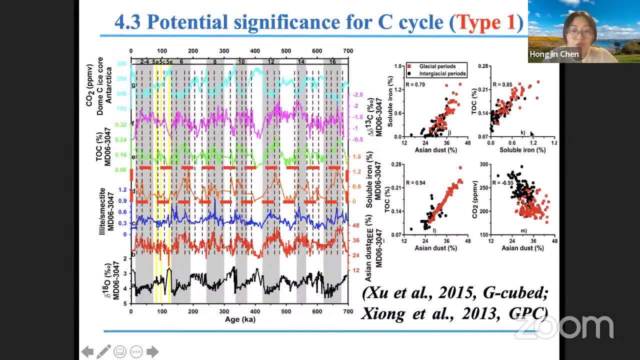 relatively good correlation between the Asian dust input, soluble ion concentration, local marine productivity and even the global atmospheric carbon dioxide concentration over the entire study interval, And also previous studies have suggested that the blooming of the diatom in the East Philippine Sea during the LGM stage would contribute to at least 1.3% of the. 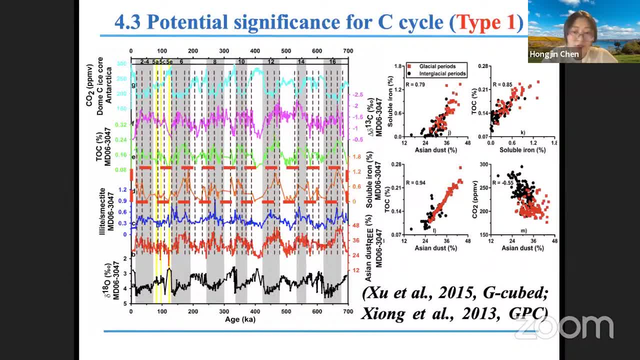 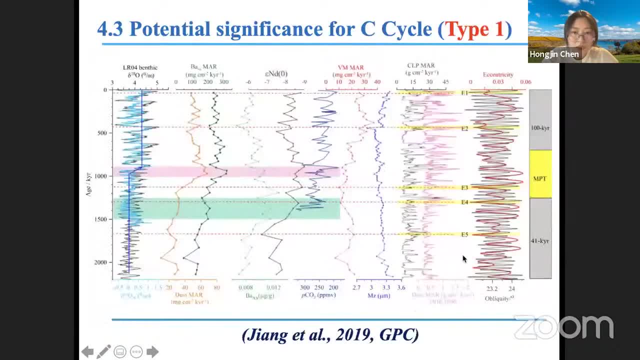 global carbon dioxide flux to the sea at this time, with only 0.08% of the seabed area, And besides, the sediment core covering a longer time period in the Eastern Philippine Sea also revealed a coupling between the flux of the eolian dust and the exported production and atmospheric CO2, further indicating that 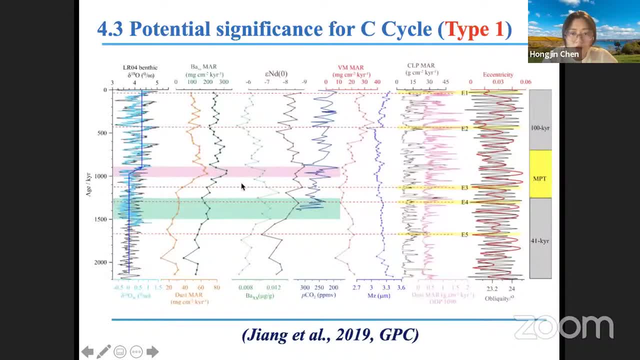 increased Asia-derived carbon dioxide concentration. So here, based on this observation, we suggest that strengthening of the biological bump induced by the enhanced input of eolian dust in the Philippine Sea and elsewhere in the tropical western Pacific during the middle to late-quaternary glacial periods may contribute to the 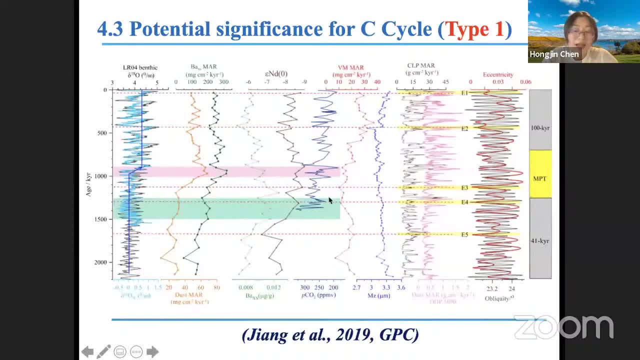 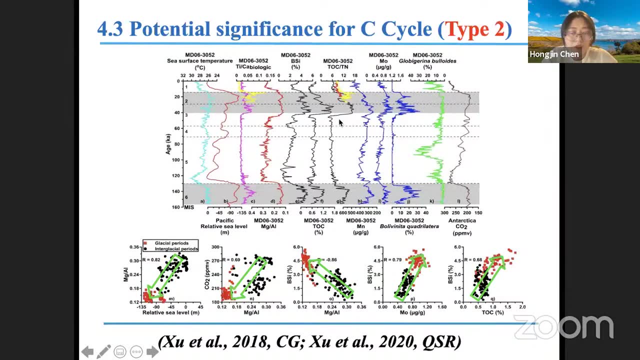 lowering of the atmospheric CO2 concentration. For the second type of scenario, which refers to the sediment core MD3052, located on the continental slope, the exposed continental shelf surrounding the tropical volcanic arcs and islands during the glacial sea level low stand might play a more important role in the global carbon cycle. 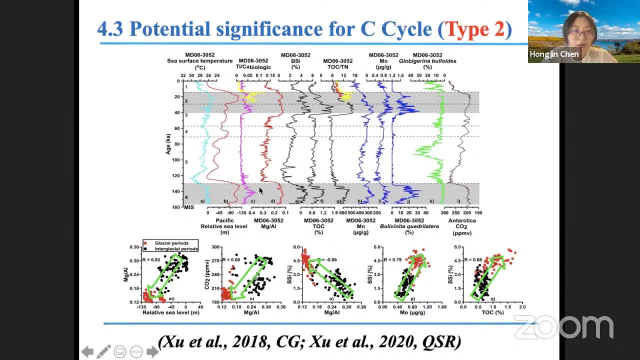 So, combined the chemical weathering and physical eolian proxies with the multi- surface temperature, sea level change and carbon dioxide concentration, a prominent feature of our record is the significant increase in both erosion and weather intensity during the MIS-6 and MIS-2 and the latter stage of MIS-3, which contrasts with many observations previously. 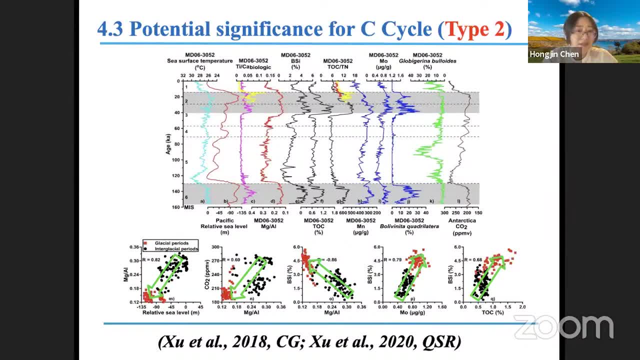 recognized in the middle latitude area and some low latitude area. This, the large sea level, low stand and associated exposure of the continental shelf in the western Philippine Sea during these cold intervals would favor the weathering and erosion of the exposed unconsolidated sediments in the shelf, which further give rise to the increased regional 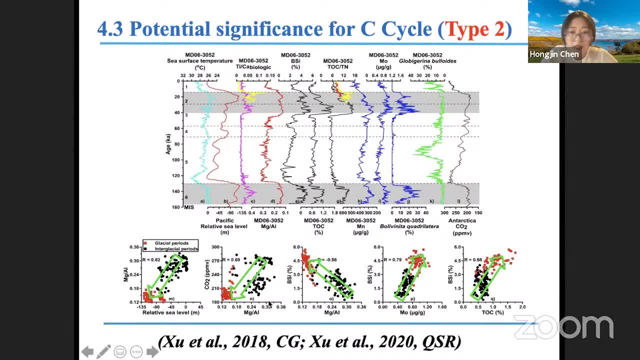 organic matter input and productivity and, in turn, decrease of the bottom water oxygenation and atmospheric CO2 concentration. The significant correlation among the chemical weathering intensity, relative sea level CO2 concentration and the productivity and organic carbon by burial further confirm this hypothesis. 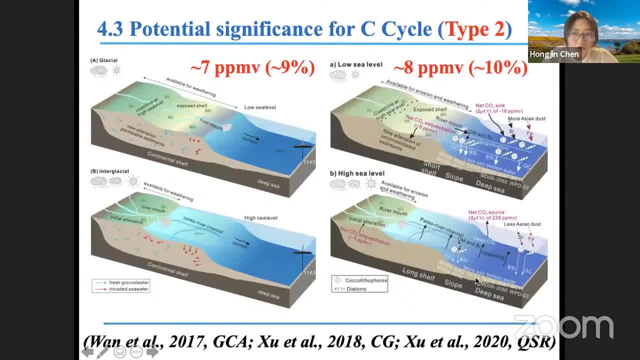 Here shows the schematic model for the process associated with the sediments available for physical erosion and chemical weathering during the glacial sea level, low stand and interglacial high stand conditions. Here shows the schematic model for the process associated with the stage on the experiment. 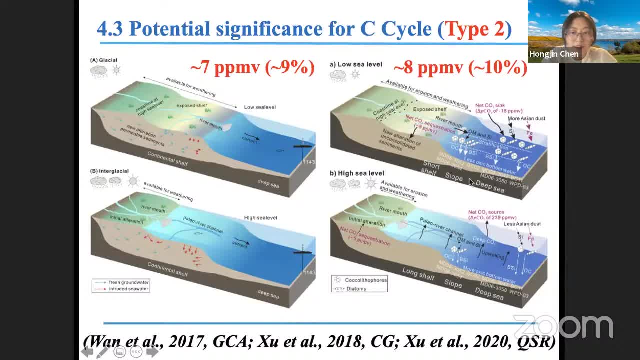 Both in the shelf around the Philippine Sea as well as the South China Sea. Simply speaking, we propose that during the quantful, sea level lows enhance chemical weathering of the exposed consolidated sediments on the tropical continental shelf, such as the South China Sea, and the tropical volcanic arcs, such as the Philippine Islands in the western Pacific. 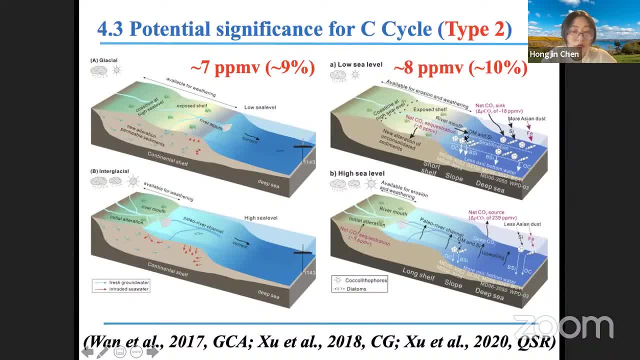 Pacific could significantly contribute to the lowering of the atmospheric CO2 concentration during the ice age. The consumption of CO2 by syndicate weathering of Luzon and the South China Sea shelf sediments during the glacial periods are estimated to be about 1.25 and 0.81 more per kilogram, which accounts for about 10% and 9% of the total. 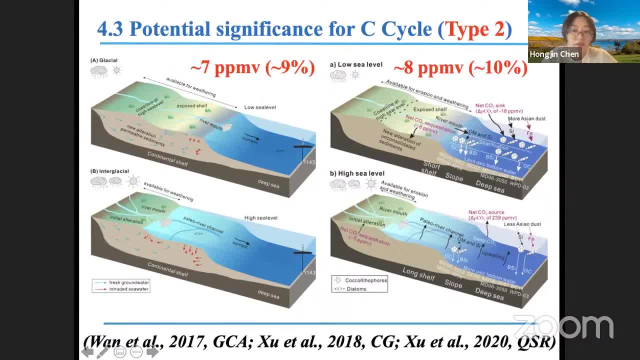 atmospheric CO2 drawdown respectively. Actually, this value is much higher than the present Himalayan weathering efficiency, which is estimated to be about 0.17 to 0.23 more kilograms. That's confirming that the weathering of the exposed shelf sediments is a more efficient 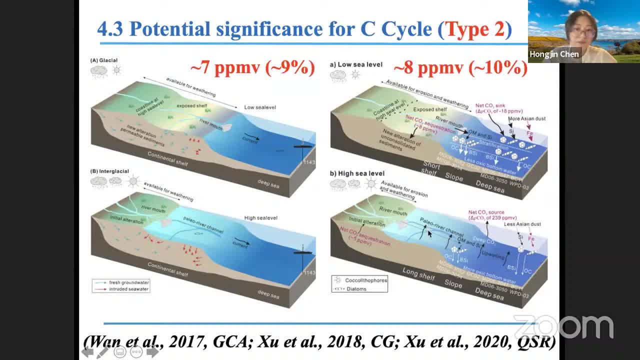 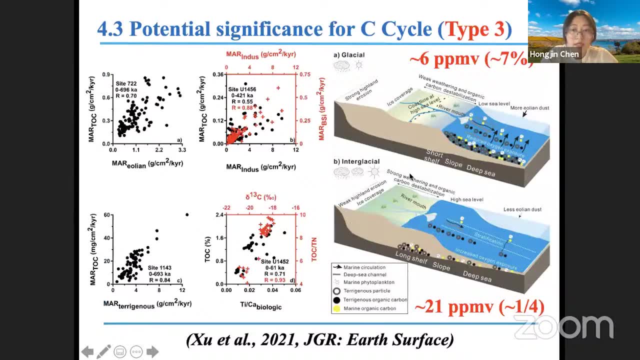 process for consuming carbon dioxide. As for the third scenario, which refers to the sediment core from the Luzon and the South China Sea, shelf sediments during the glacial periods, the Arabian Sea, together with representative core from the Bay of Bengal, enhanced burial of. 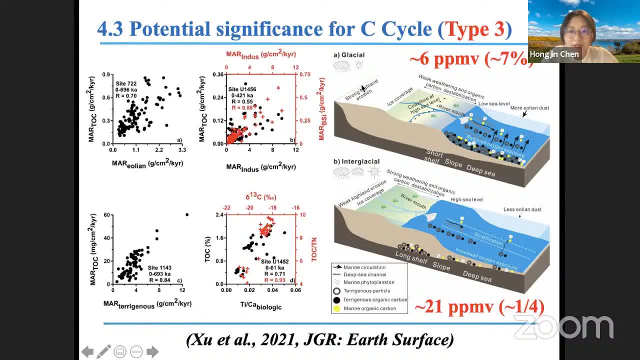 organic matter dominantly sourced from the highlands syndicate erosion, also play an important role in the global carbon cycle. So, by comparing to the high-resolution comprehensive sediment records of many high-quality sediment core profile in the Eastern Indian Ocean, as well as the 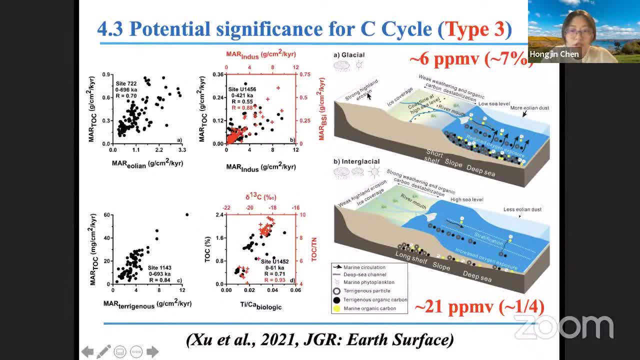 South China Sea shelf sediments. we can see that the high-quality sediment core profile in the South China Sea shelf sediments is a more efficient process for consuming carbon dioxide. We found that during the quaternary glacial periods, physical erosion in the high altitude. 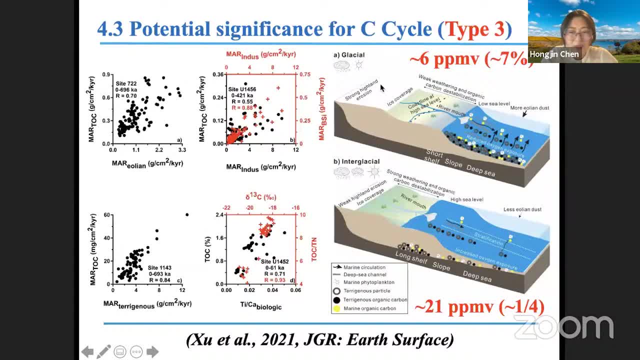 areas of the Himalaya and the Tibetan Plateau, which brought a large amount of terrestrial detritus, nutrients and organic matter to the study area, thus in turn stimulate the biological productivity, the development of the anoxic condition on the seafloor and the increase of 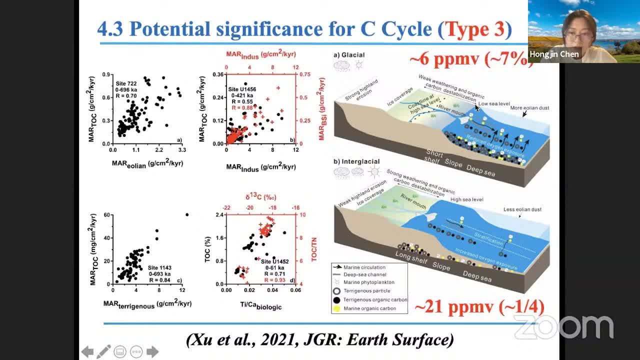 the burial flux of organic carbon In the case of the high-resolution sediment, both derived from the sea surface productivity or from the terrestrial input on the seafloor. this hypothesis can be further confirmed by the significant correlation between the burial of organic carbon and eolian dust concentration in 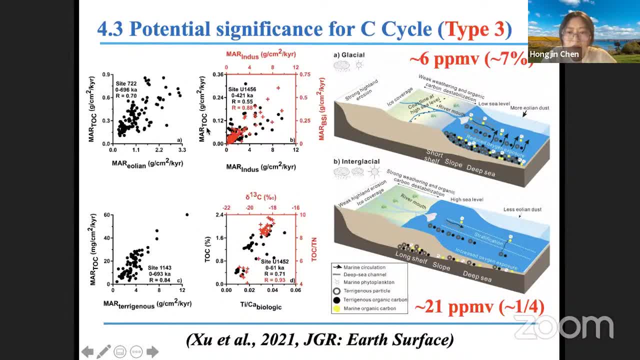 the Western Arabian Sea and the terrestrial input from the Himalaya and Tibetan Plateau and the terrestrial detritus from the continental shelf in the South China Sea. This process, associated with physical erosion in the Himalaya and Tibetan Plateau and transport to the produced detritus and organic matter, would explain about 7% of the atmospheric CO2. 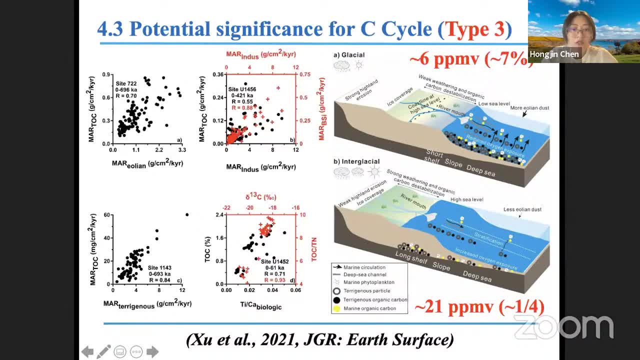 concentration drawdown during the quaternary ice age. So, in summary, during the low sea level stage of the quaternary ice age and the increased chemical weathering of the silicate sediments on the sea surface, the chemical weathering of the 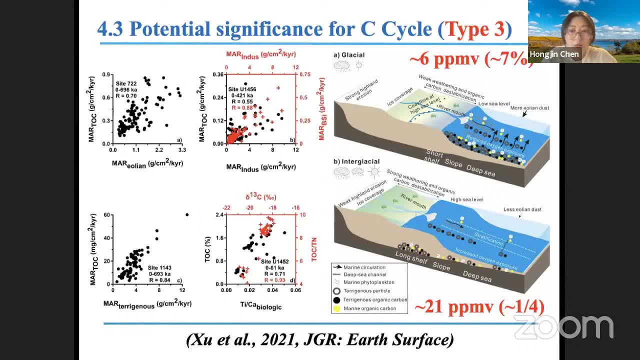 surface caused the tropical content in the shelf, like South China Sea, Western Philippine Sea, together with the strength and silicate physical erosion in the Himalaya and Tibetan highlands. The activity of deep-sea channels stimulated marine productivity and large-scale burial of organic carbon in the tropical marginal sea, like the distant Arabian Sea, Bay of Bengal, South China Sea, made those areas an important contributor to the modulation of the surface. 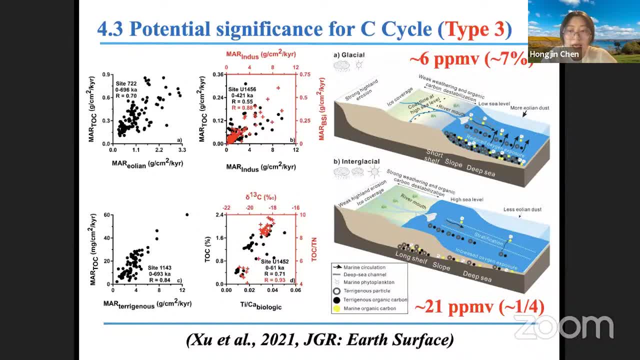 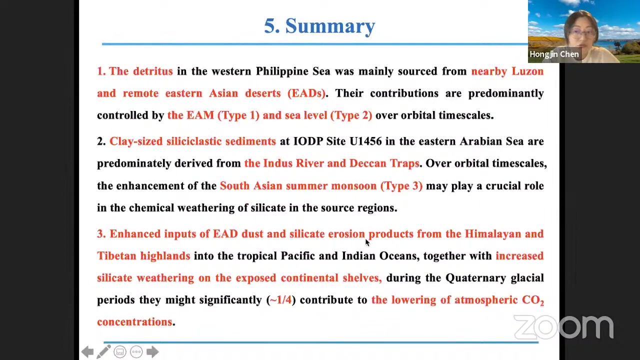 To be continued, of global organic carbon preservation and the atmospheric CO2 concentration. So altogether, this process would account for about a quarter of the total decrease in the atmospheric CO2 concentration during the glacial periods. So, in summary, several major conclusions have been drawn. 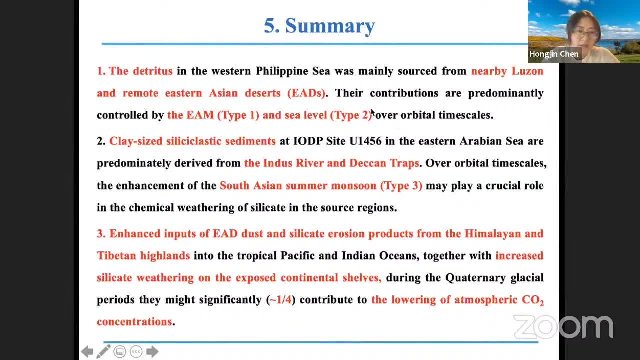 here for the type one and type two sediment tramps, or the modern sediment tramps or the sediment core. The detritus in the Western Philippine Sea was mainly sourced from the nearby and remote Asian deserts. Their contributions are predominantly controlled by the East Asian monsoon and the sea level change. 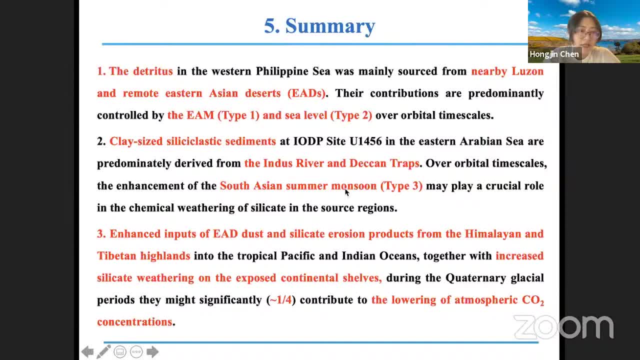 over orbital timescales. For the type three sediment core, the clay-sized silicic plastic sediments from the IODP site in the Eastern Arabian Sea are predominantly derived from the Indus River and the Deakin Tramps Over orbital timescale. 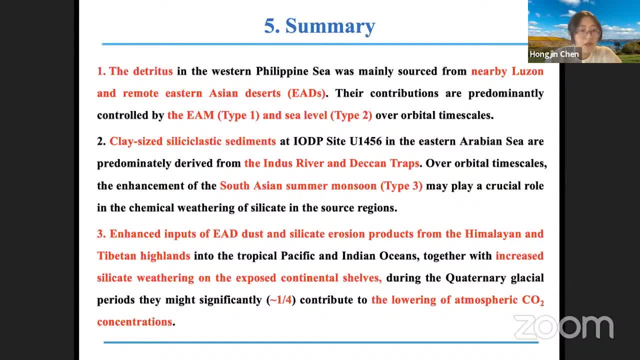 the enhancement of the South Asian summer monsoon may play a very important role in the chemical weathering of silicates in the source region. So altogether, the enhanced input of Eastern Asian desert dust and silicate erosion products from the Himalaya and Tibetan highlands. 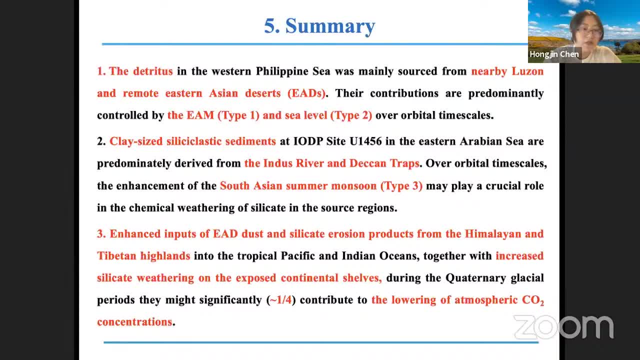 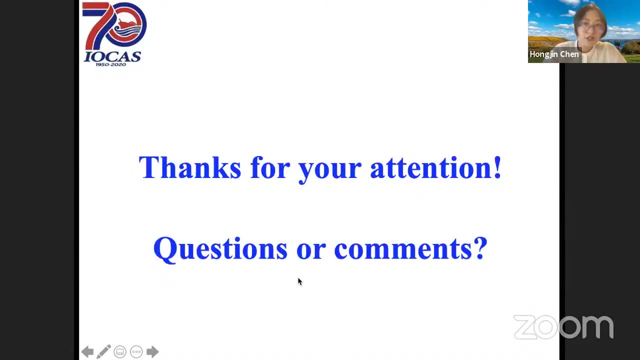 into the tropical Pacific and Indian Ocean, together with increased silicate weathering on the exposed continental shelf during the continental glacial periods, might significantly contribute to the lowering of the atmospheric CO2 concentration. That's all for my presentation. Thank you so much. 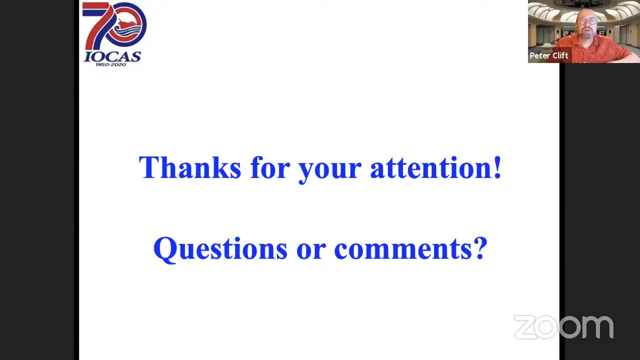 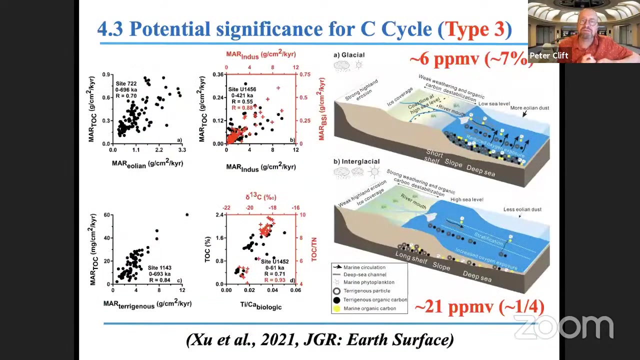 Thank you very much. Thank you. Thank you for your time, So are there any questions from the audience? I'd like to ask a question. So you were talking about the organic matter content of the sediments and the fact that the organic material 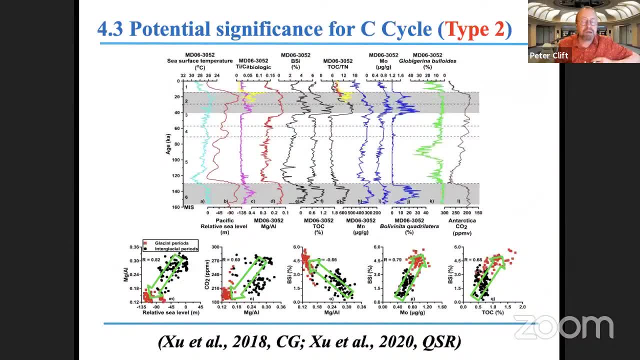 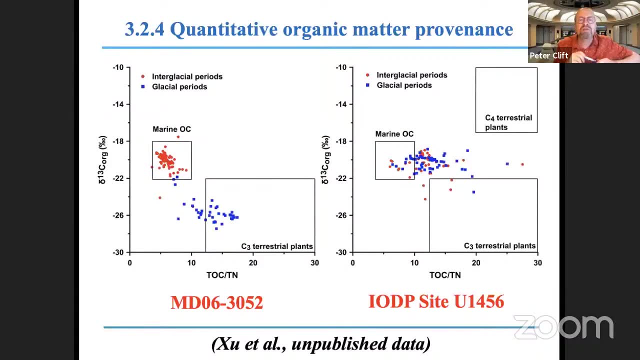 was coming from different sources in the past, during glacial and interglacial cycles, And especially more, I think it was more organic material. Yes, like this type of thing, Exactly So. but So the source of the organic material is changing. 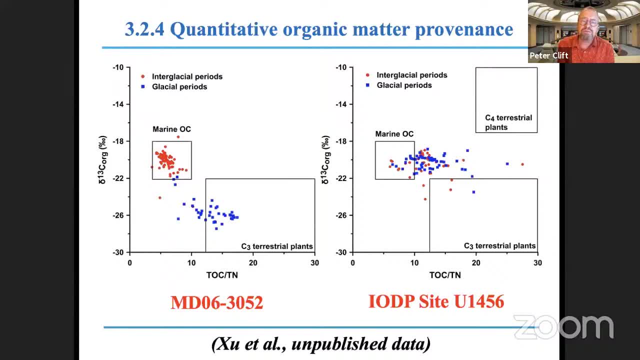 but I wondered if the total flux was also changing, because that would be dependent on the volumes of sediment that were being deposited in the deep ocean. Can you factor that in to look at the volumes of material rather than just- I mean the source of the organic matter is changing. 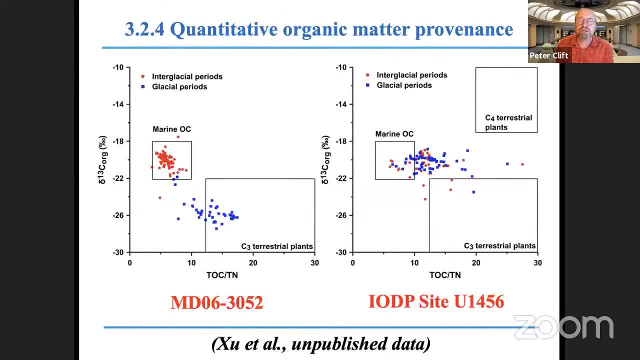 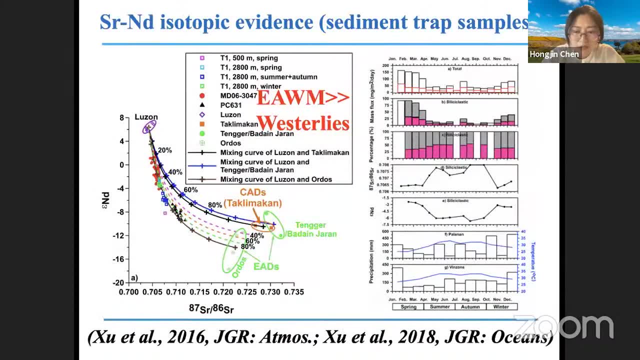 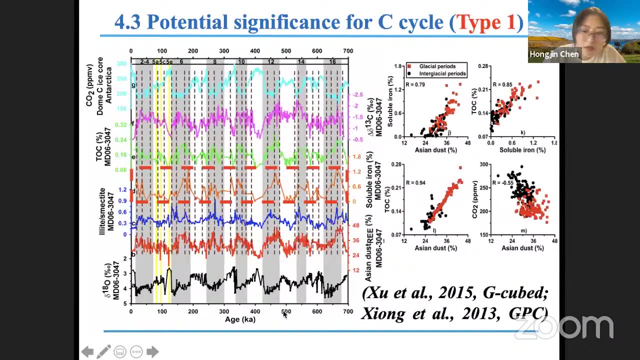 but do we know if the total amount is changing? Okay, okay, Actually we did calculate the mass accumulation rate of the total organic carbon. I'm not sure if I, Maybe it's not showing this. Yeah, But we actually, yeah, calculate for the sediment core. 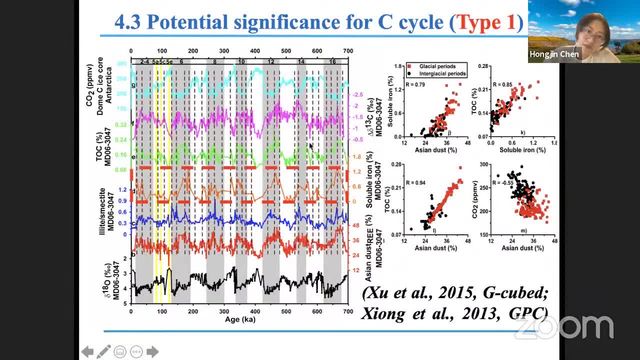 like I believe maybe, Yeah, Yeah, Maybe it's 3047 or 3052, we would calculate And it shows very good the glacial and interglacial cycle over the orbital time scale and with increased mass accumulation rate of the total organic carbon during the glacial periods. 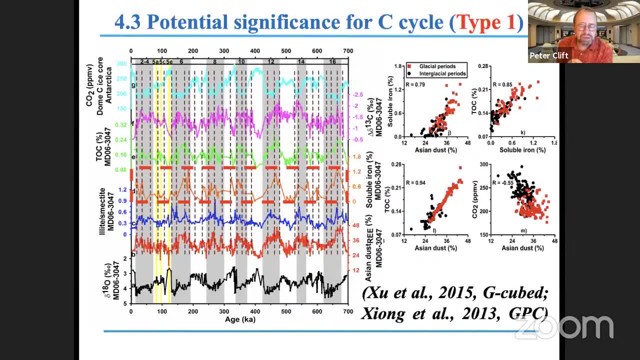 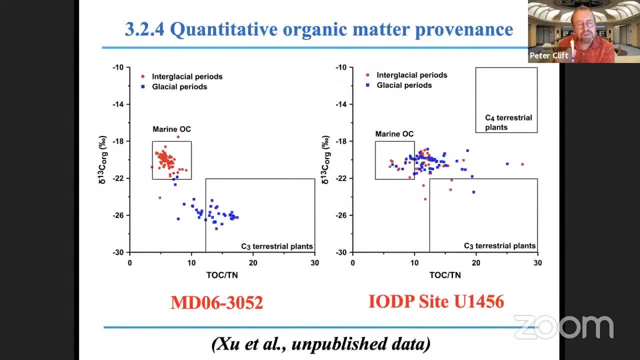 Right, Actually, because that was sort of. that was what I was wondering, I guess, Because one thing that we've seen in the Arabian Sea is that a lot of the sediment that's deposited during the glacial time is actually originally eroded. 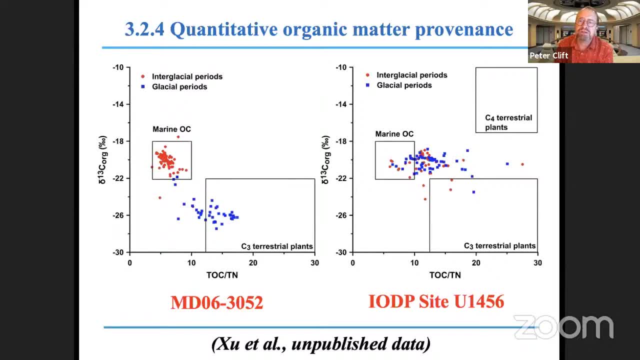 during the interglacial time And it's stored on the continental shelf and in the floodplains and then redeposited during the glacial time. But perhaps that doesn't affect the organic matter so much, because I mean it might be difficult. 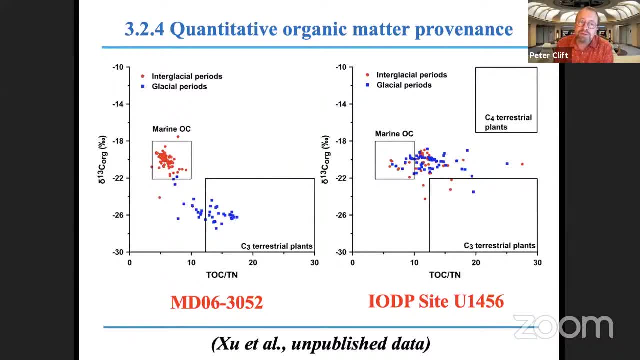 to store organic matter on floodplains without it oxidizing. So presumably the organic matter deposited during the interglacial times would be fresh, would be new material, I wonder. Okay, One other question I had was: so you were talking about the carbon impact. 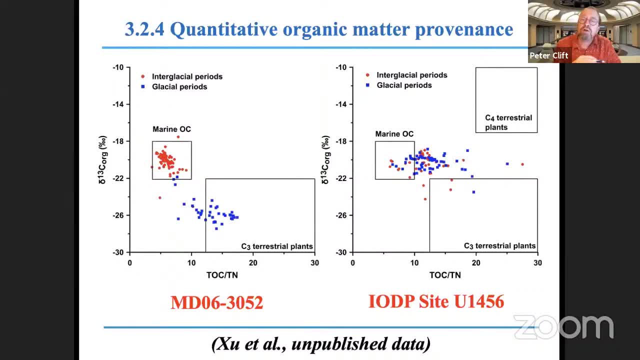 the impact on the carbon budget of weathering, chemical weathering, on the exposed continental shelf And I wondered: is there a way to estimate the impact of what happens to the growth of forests on these exposed shelf? Presumably that would also draw down CO2. 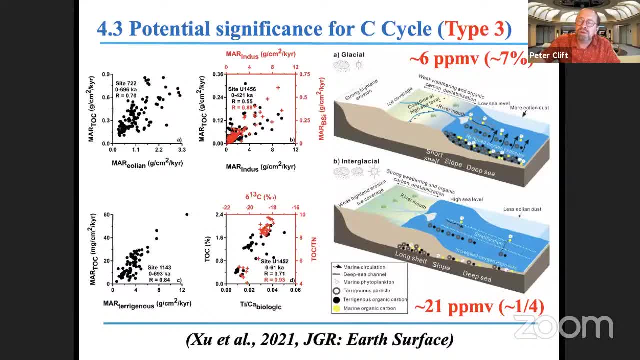 during the glacial time? Do we know the relative impact? Do we know the importance of vegetation growth compared to chemical weathering in controlling the CO2 during the glacial interglacial cycles? You see what I mean. Okay, I'm not sure about if we 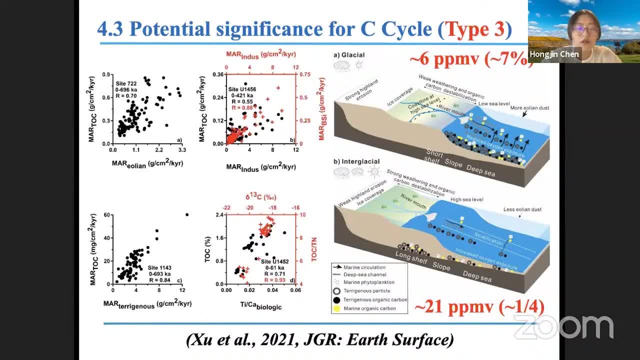 I think maybe we didn't take into consideration of the vegetation during the glacial and interglacial periods And I think maybe during the glacial periods and the vegetation would be more, less And, yeah, it would act in the contract way to the CO2 concentration. 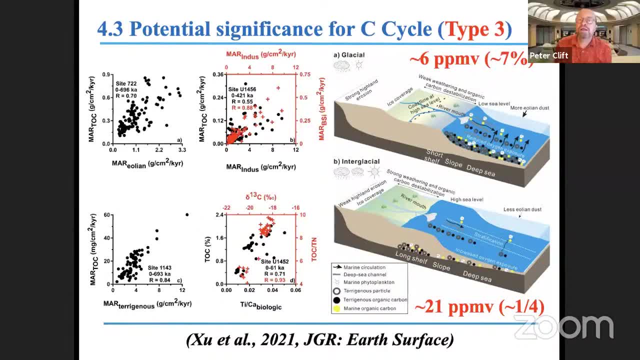 Right, So we didn't take that into consideration. I guess it would help you, though. right, Because you would have. you're consuming more CO2 because of chemical weathering of the shelf, But you also taking carbon out of the atmosphere to grow a forest on these low latitude shelves. 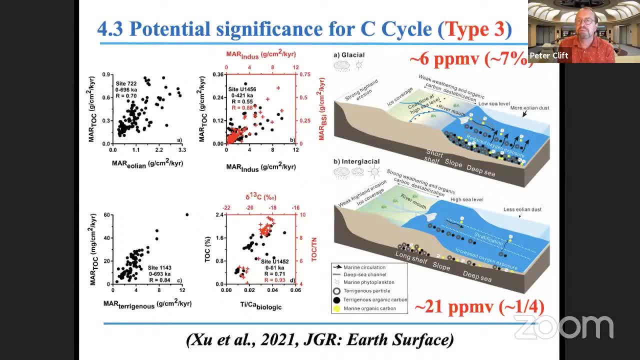 It would make the effect stronger, I would guess, but maybe, Okay, Okay, Yeah, that's that would be my guess. Yes, it's a very interesting view, And maybe we'll take that into consideration in the future. Yeah, I'm not entirely sure. I have to do it myself.